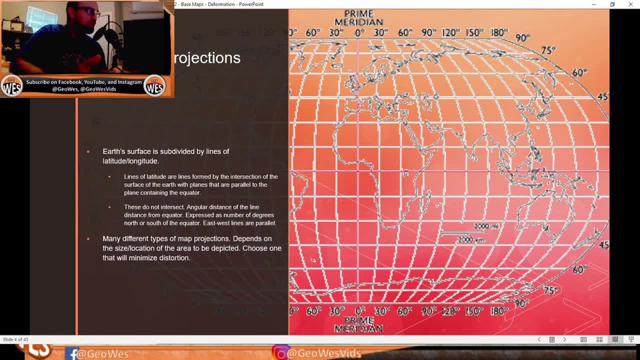 subdivided by lines of latitude and longitude. Lines of latitude are lines formed by the intersection of the surface of the earth with the planes that are parallel to the plane containing the equator. It's kind of confusing how the book puts it, but lines of latitude are just these lines going from east to west. These do not intersect. Angular distance of the line, distance from the equator, is expressed as number of degrees: north or south. north or south of the equator. 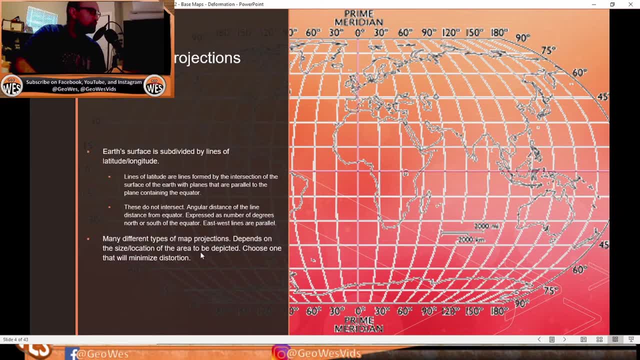 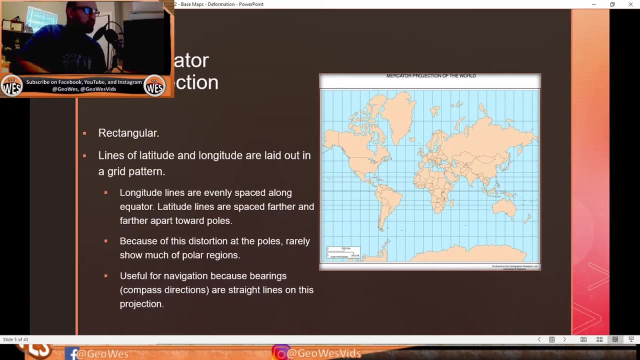 The east-west lines are parallel. Many different types of map projections. It depends on the size and the location of the area to be depicted. Choose one that will minimize the distortion. So this is the first projection. It's called the Mercator projection. It's rectangular. As you can see, all these lines of latitude and longitude create either long rectangles or perfect squares near the equator. 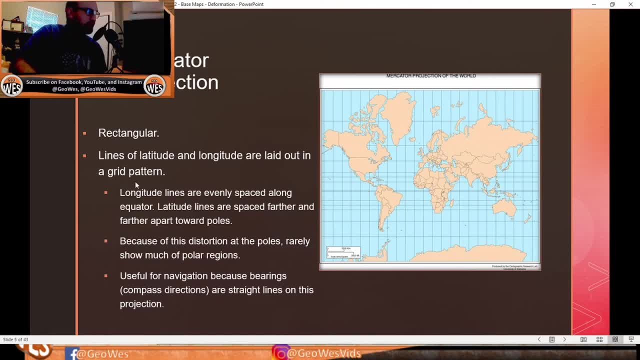 Lines of latitude and longitude are laid out in a grid pattern. Longitude lines are evenly spaced, As you can see, all pretty much evenly spaced. What changes is the latitude? They're spaced further and further, apart from the poles, And you know, the maximum distance between lines of latitude are up here And then, once you get to the poles, they're closer together. 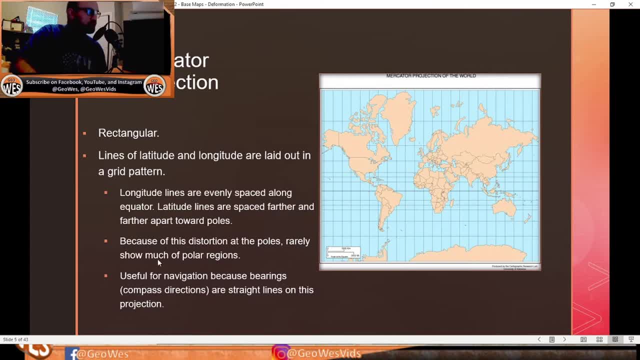 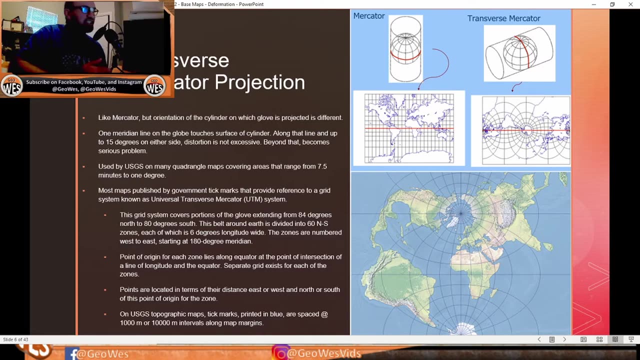 And because of this distortion at the poles it's rarely used. It's rarely used to show the polar regions. It's useful for navigation because bearings or compass directions are straight lines on this projection. And then we have the transverse Mercator projection: Like the Mercator, but the orientation of the cylinder on which that's supposed to be globe is projected as different. 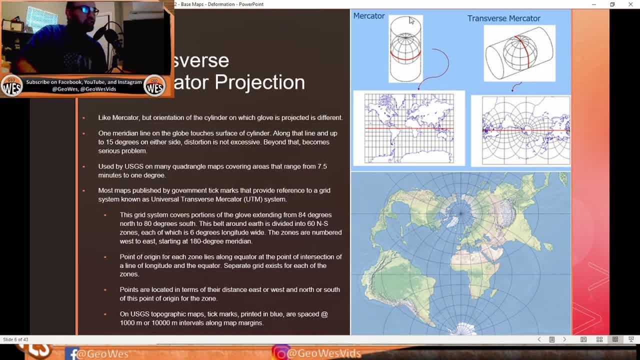 As you can see, the Mercator, the cylinder, is basically parallel With the globe, whereas the transverse Mercator is transverse to the to the globe. So one meridian line on the globe touches the surface of the cylinder, as you can see here, along that line and up to 15 degrees on either side. 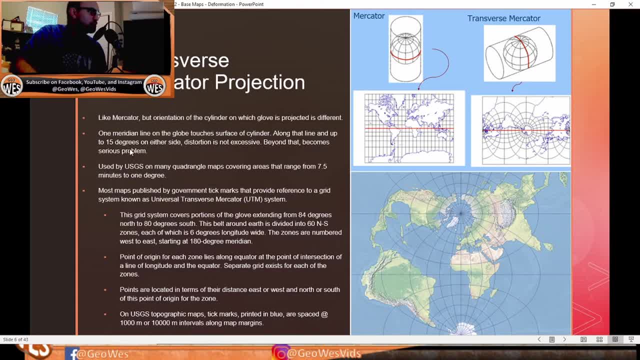 The distortion is not excessive. Beyond, that becomes a serious problem. It's used by the USGS on many quadrangle maps covering areas that range from 7.5 minutes to one degree, But a liquid transfer of coverage would still be useful. The Earths' grid system, or tremorURT, is a chỉing beam. 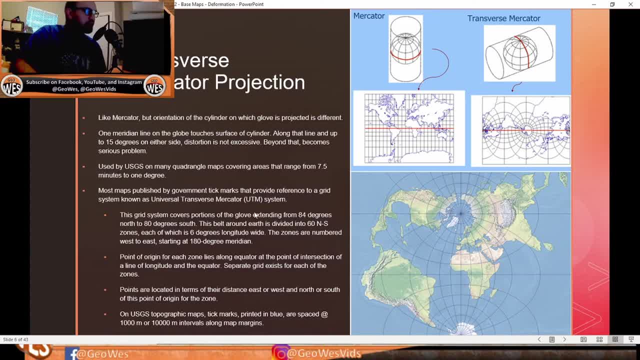 It's created thanks to quería frontalioned maps published by government tick marks that provide reference to a grid system known as the universal transverse Mercator system. This grid system covers portions of the globe extending from 84 degrees north to 80 degrees south. 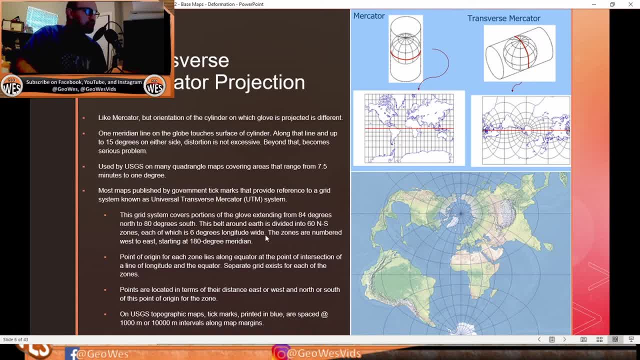 This belt around the Earth is divided into 60 north-south zones, each of which is 6 degrees longitude wide, numbered west to east. The point of origin for each zone lies along the equator, at the point of intersection of a line of longitude and the equator. 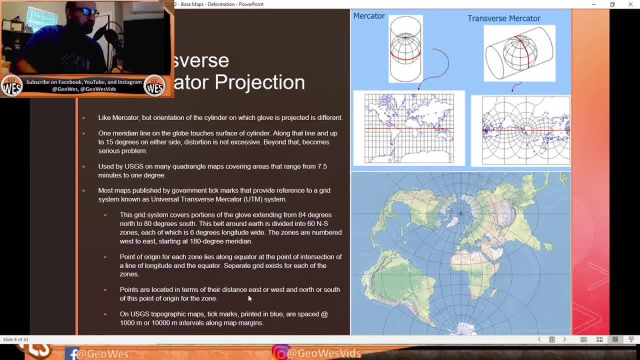 Separate grid exists. Points are located in terms of their distance: east or west and north or south of this point of origin. for the zone On USGS topographic maps, tick marks printed in blue are spaced at 1,000 or 10,000 meters meter. 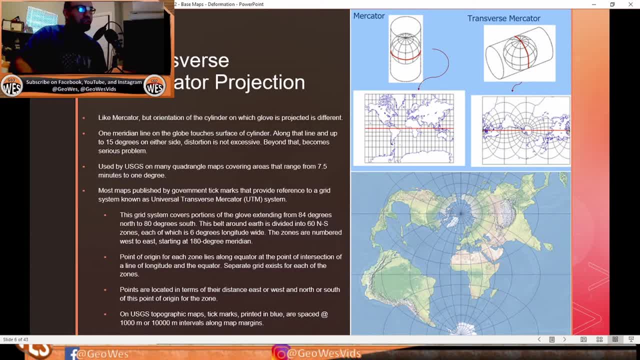 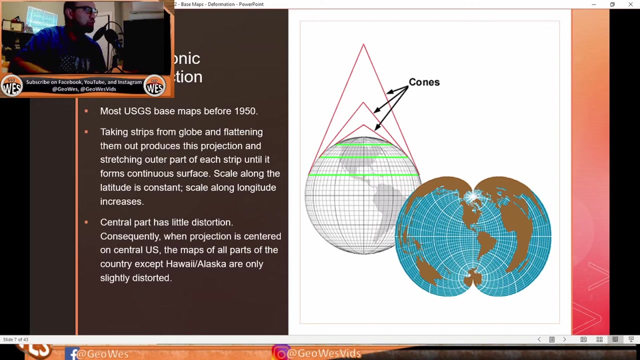 intervals along the map margins And you can see the difference in how they're projected. You know this looks normal and distortion is going to be worse away from this red line and this transverse Mercator projection. And this is another way to visualize it. So the polychonic projection. most USGS basemaps used this. 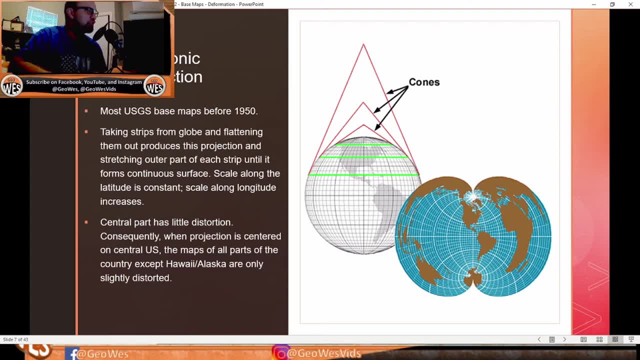 projection before 1950.. Take a look at this. Take a look at this: Taking strips from the globe and flattening them out produces this projection and stretching and it stretches the outer part of each strip until it forms a continuous surface. The scale along the latitude is constant. The scale along 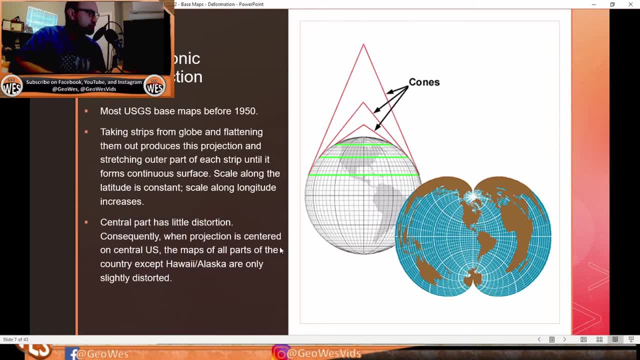 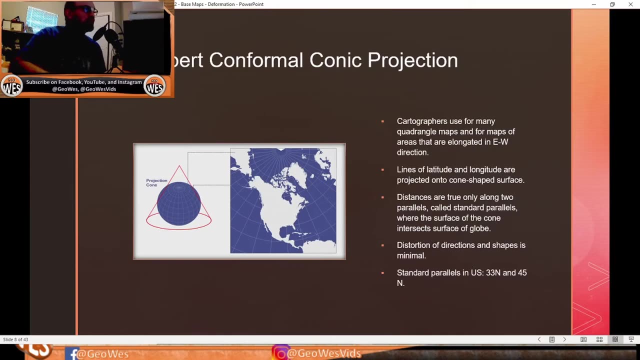 longitude increases, The central part has little distortion. Consequently, when projection is centered on the central US, the maps of all parts of the country except Hawaii and Alaska are only slightly distorted. The Lambert conformal conic projection Cartographers use this projection for many quadrangle maps. 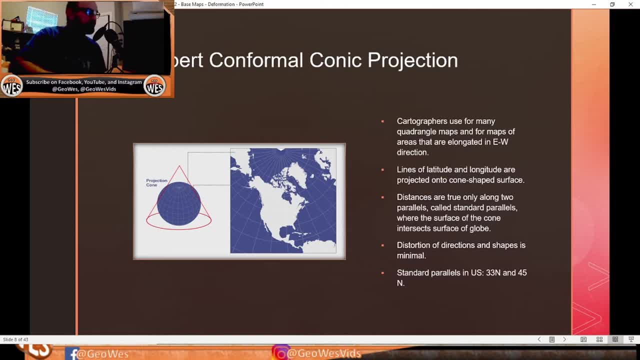 and for maps of areas that are elongated in the east to west direction. Lines of latitude and longitude are projected onto a cone-shaped surface. Distances are true only along two parallels, called standard parallels. where the surface of the cone intersects with the surface of the globe, Distortion of the directions and shapes is minimal. The standard 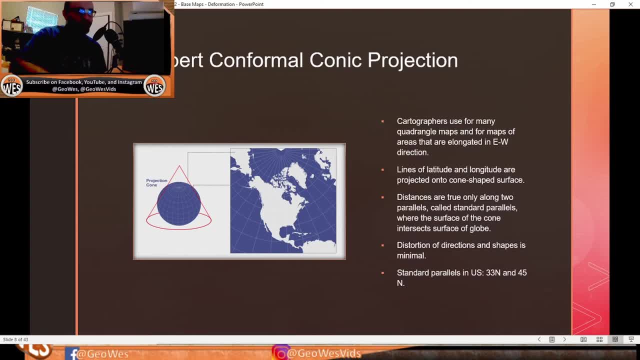 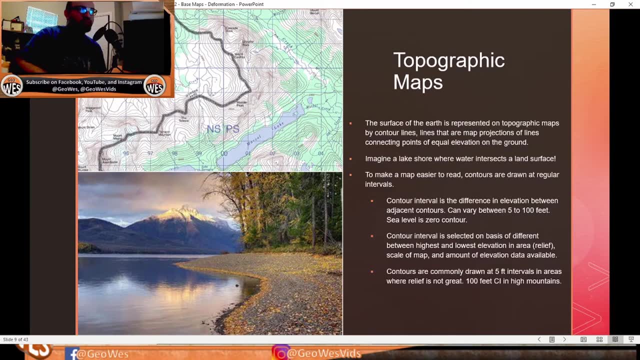 parallels in the US are 33 north and 45 north. So topographic maps. The surface of the earth is represented on topographic maps by contour lines, Lines that are map projections of lines connecting points of equal elevation on the ground. Imagine a lake shore, as you can see on the bottom left picture. We're going to. 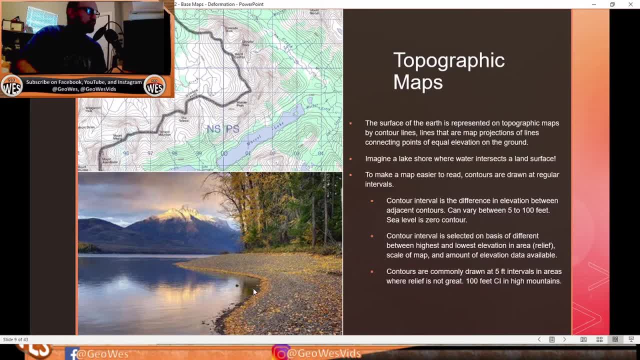 draw a map of the lake shore where the water intersects a land surface. So right here, And that would represent a contour line, if you can visualize that. To make a map easier to read, contours are drawn at regular intervals. The contour interval is the difference in elevation. 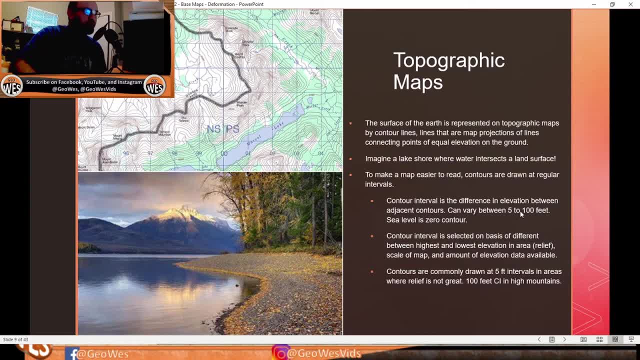 between adjacent contours. It can vary between 5 to 100 feet. Sea level is obviously the zero contour. Contour interval is selected on the basis of difference between the highest and lowest elevations in the area. It's called relief, The scale of the map, the amount of 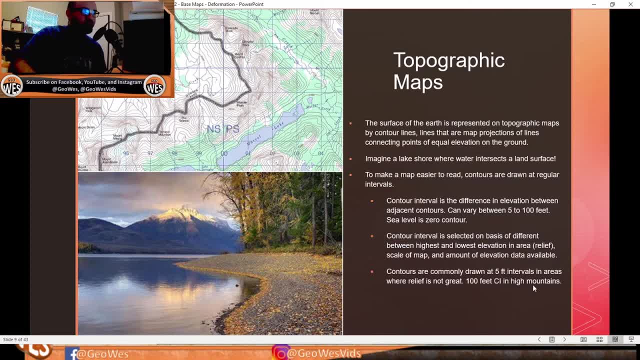 elevation data available. Contours are commonly drawn at 5 foot intervals in areas where relief is not great And a 100 foot contour interval in high mountains. So let's see Contour interval for this one is what? 20? 20 contour interval for this topo map right here. It's good to 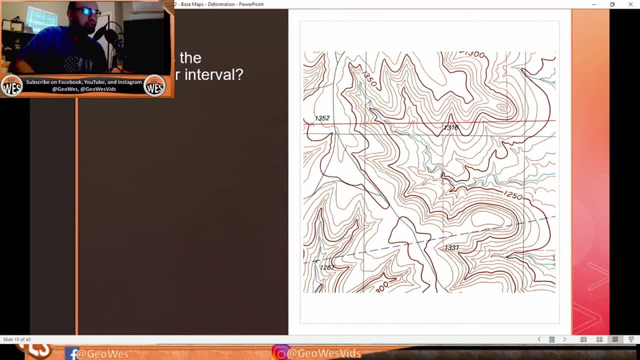 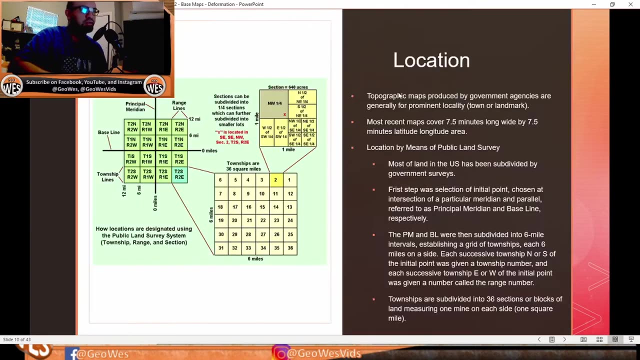 practice. Okay. so what's the contour interval for this one? So let's see, This is their 1300.. One, two, three, four, five. Difference is 50.. So that's about 10 foot contour interval. 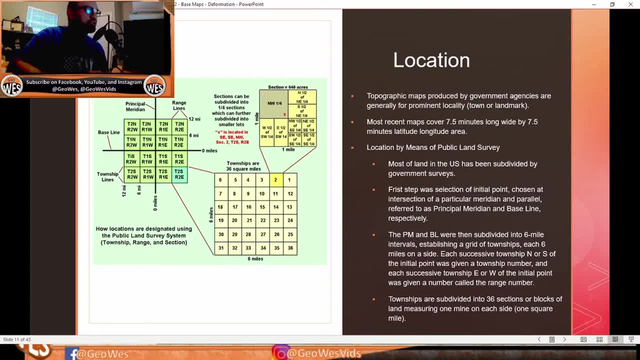 Okay, the location. The topographic maps produced by government agencies are generally for prominent locality, town or landmark. Most recent maps cover 7.5 minutes long wide by 7.5 meters wide. minutes latitude, longitude area location by means of public land survey: most of 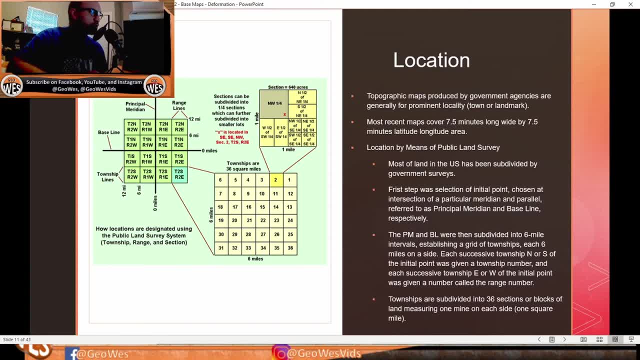 the land in the us has been subdivided by government surveys. the first step was the selection of initial point chosen at the intersection of a particular meridian and parallel- so that would be right here- referred to as the principal meridian and the baseline, respectively the PM. 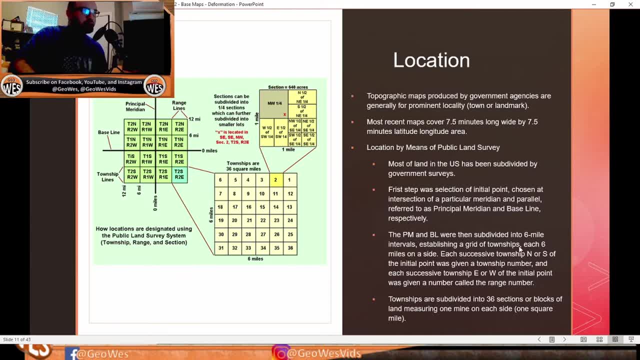 well. the prime meridian and the baseline were then subdivided into six mile intervals, establishing a grid of townships each six miles on a side. each successive township north or south of the initial point was given a township number, and each successive township east or west of the initial point was given a. 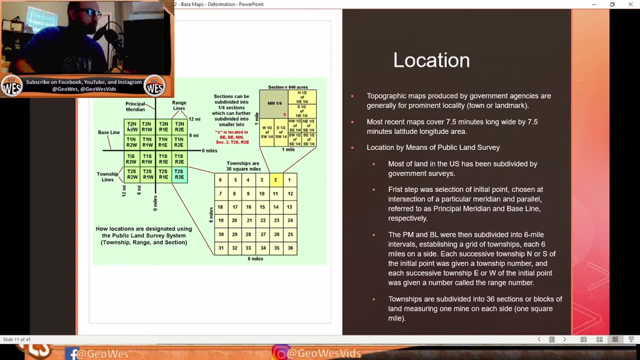 number called the range number and, as you can see, you know you have your township number and your range number and all these little squares. townships are subdivided into six mile intervals each six mile intervals. each township are subdivided into 36 sections or blocks of land measuring one mile on. 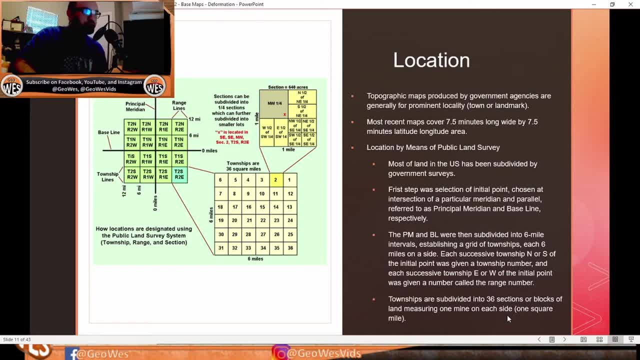 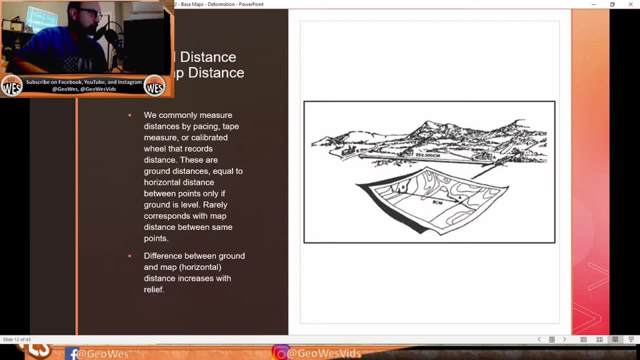 each side- not mine, man, I have a lot of typos- which is called this one square mile. so ground, ground distance and map distance. we commonly measure distances by pacing tape measuring or calibrated will that records distance. these are ground distances equal to the horizontal distance between points only if the 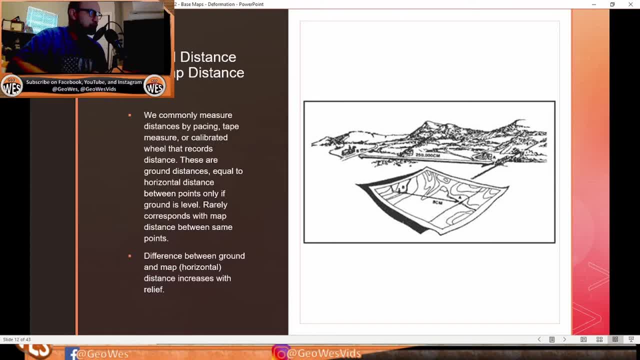 ground is level rarely corresponds with map distance between the same points, unless the ground is very flat, high terrain areas. it's gonna. that's gonna change. you know the the ground distance and map distance, the variations between the two, so the difference between the ground and map, or 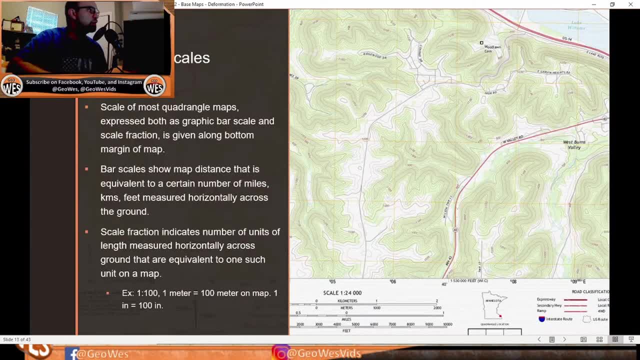 horizontal distance increases with relief map scales. scale of most quadrangle maps, expressed both as a graphic bar and a scale fraction, is given along the bottom margin of the map, as you can see right here in each of the map, as you can see right here in each of the map, as you can see right here in. 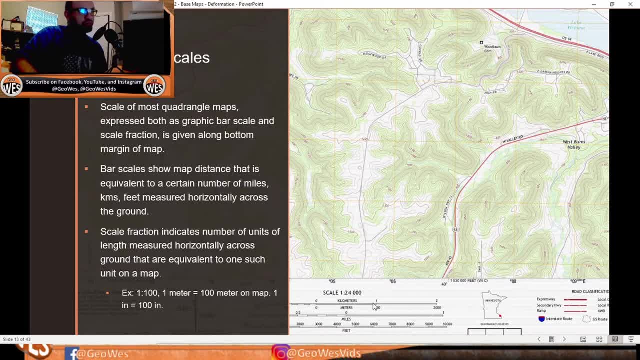 And you actually have three different ones, for if you want to use kilometers, meters, miles or feet, Bar scales show the map distance that is equivalent to a certain number of miles, kilometers, feet measured horizontally across the ground. Scale fraction indicates the number of units of length measured horizontally across the ground that are equivalent to one such unit on a map. 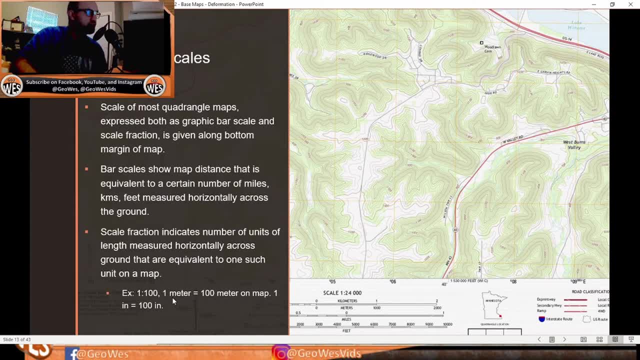 So, for example, 1 to 100 could be: 1 meter equals 100 meters on this map. Actually, this map is 1 to 24,000.. So 1 meter equals 24,000 meters on this map. 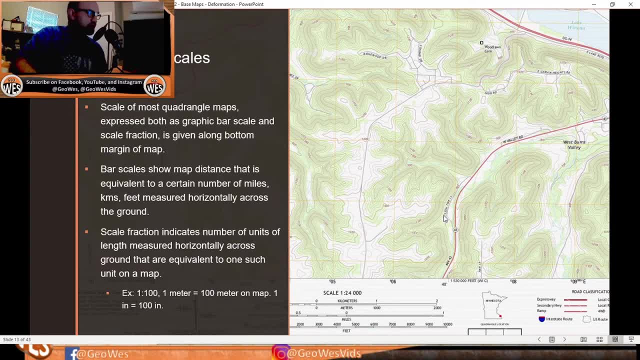 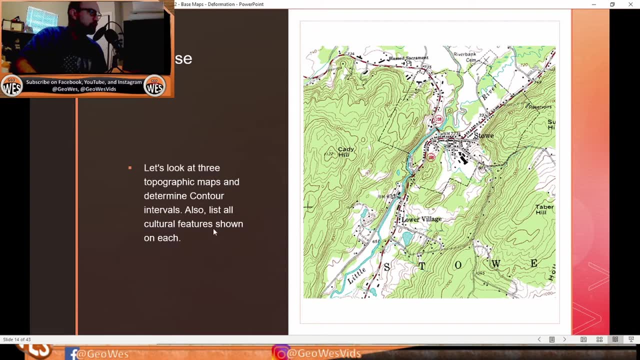 Or 1 inch equals 24,000 inches on this map. Let's look at the three topographic maps and determine contour intervals And let's list all the cultural features shown on each. Okay, so contour interval here's 900.. 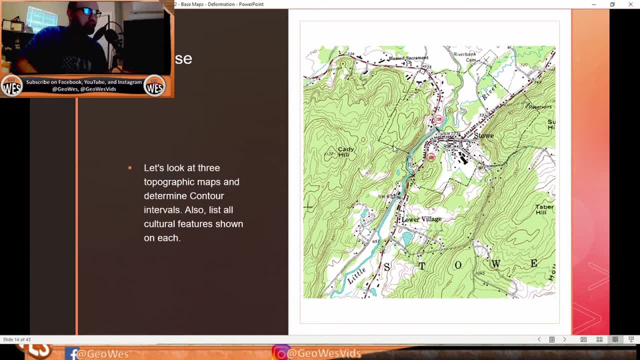 As you can see, it's bolded. That makes it one of the major topographic contours on the map, And then you have 1,000.. So let's count the lines 1, 2,, 3,, 4, 5.. 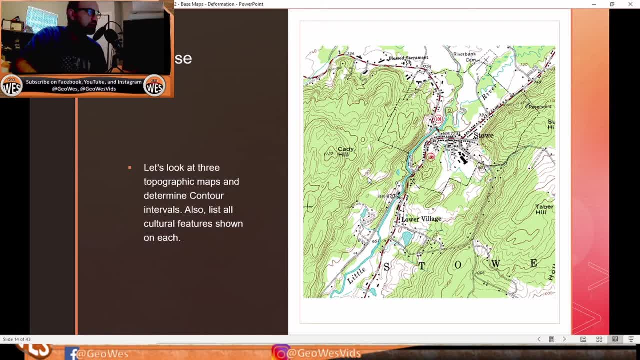 So the difference of 100.. So that's 20.. The contour interval is 20.. And in terms of cultural features, we have some roads- I am guessing this is a railway for a train. You have rivers. There's a church right here. 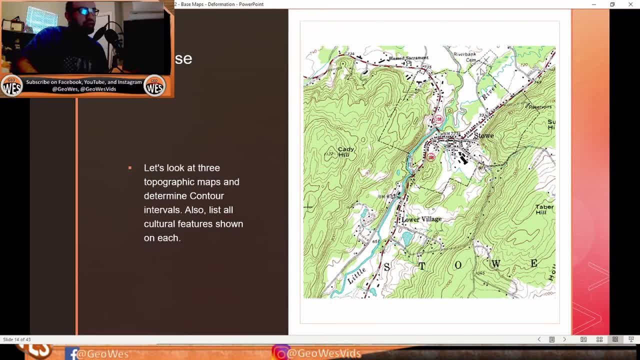 A cemetery demarcated by a cross Reservoir, probably for water, Some structures demarcated by the black squares. This one's a big building right here. Yeah, I mean, that's all I see. it looks like Okay. 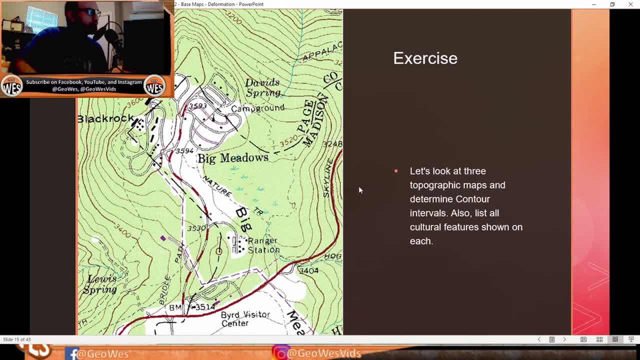 So here's another one. All right, so maybe I zoomed in a little too much on this one. All right, so we have 3,400.. Looks like it's going to be. let's see 1,, 2,, 3,, 4,, 5, 200 divided by 5.. 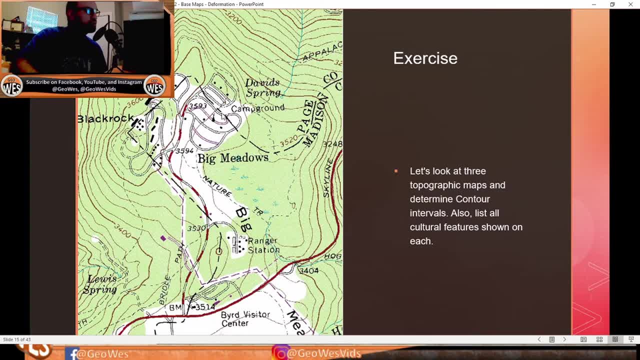 That's 40. 40-foot contour interval, And then we have a campground. We have roads. We have a railway, it looks like, Or maybe a major road. Let's see what else we got: Visitor center, A benchmark elevation right here. 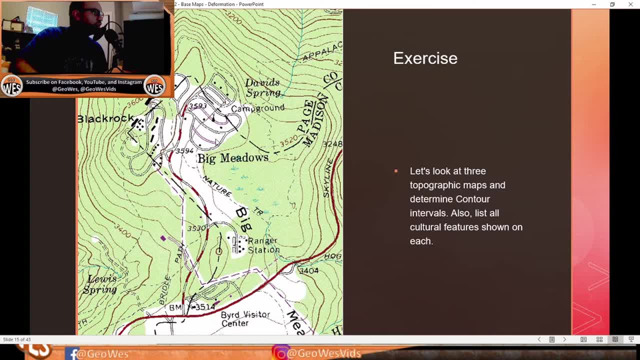 Yeah, we have structures again: Roads, An amphitheater, I'm guessing is right here- Some rivers. It looks like this is a wetland or, my doubt, a swamp, But it looks like a wetland right here called Big Meadows. 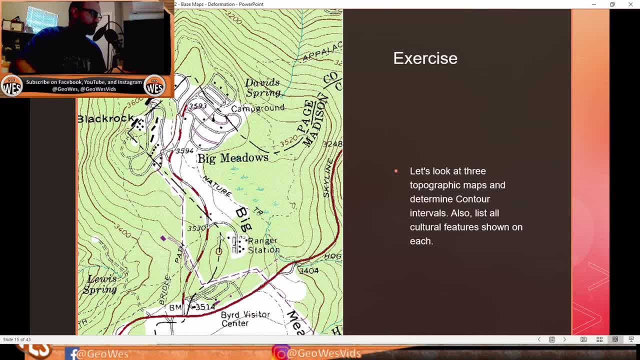 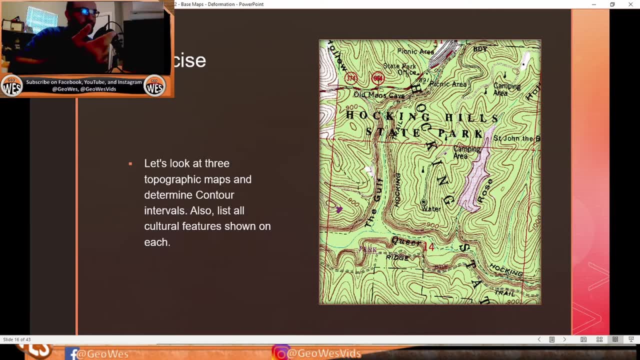 Okay, Ranger station. Oh yeah, that looks good. Okay, Let's look at. okay, let's look at this map too. Okay, so what's the contour interval? We have some steep. looks like a river valley. 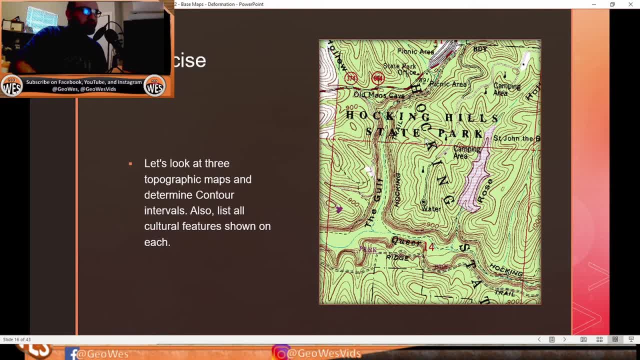 Steep right here on each side. Let's see So the contour interval we have, Okay, Okay. so this is the 900 right here: One, two, three, four, five. So it's going to be a difference of 100 divided by five lines. 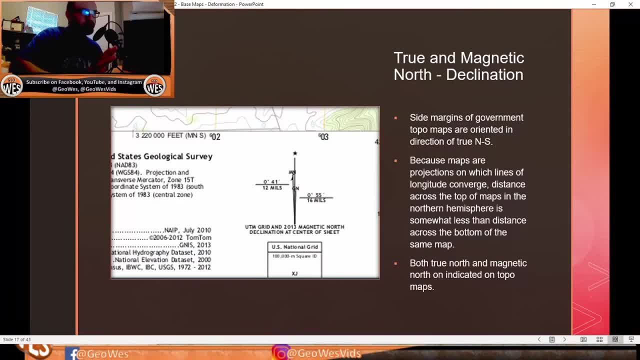 That's 20.. So a 20 contour interval, And it's good to practice that type of stuff. Okay, So true and magnetic north declination. The side margins of government topographic maps are oriented in the direction of true north-south. 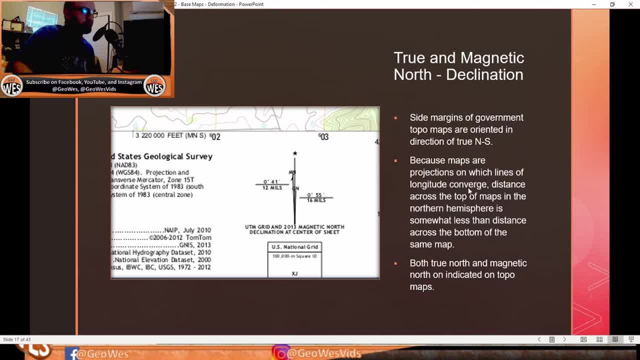 Because maps are projections on which lines have long Longitude converged. the distance across the top of the map in the northern hemisphere is somewhat less than the distance across the bottom of the same map. Both true north and magnetic north are indicated on topographic maps, as you can see with this symbols right here. 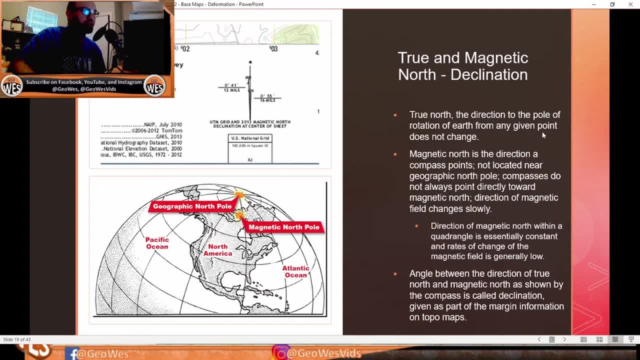 So true north. the direction to the pole of the rotation of earth from any given point does not change. So true north is geographic north And magnetic north is the direction a compass points. It is not located near the geographic north pole. 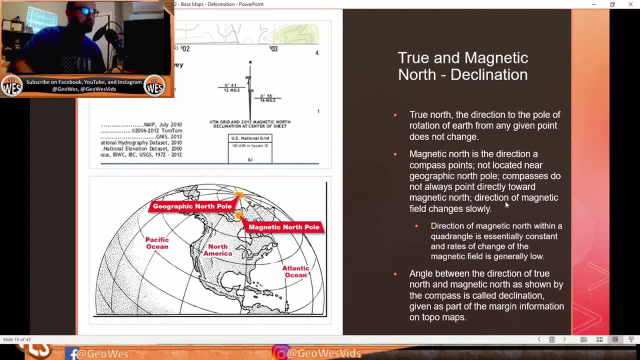 It Compasses do not always point directly toward the magnetic north. Direction of the magnetic field changes slowly. Direction of the magnetic north within a quadrangle is essentially constant And rates of change of the magnetic field is generally low. Angle between the direction of true north and the magnetic north as shown by the compass is called declination. 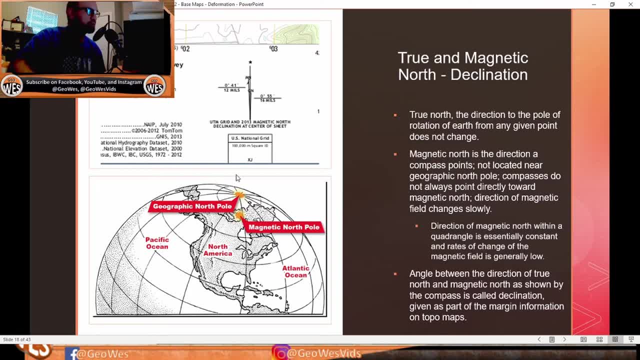 Given as part of the margin information on topographic maps. So, according to this map, Minnesota, I believe, is. So Minnesota is somewhere right here. Sorry, I'm not an expert on those states up there, But So we have Minnesota. 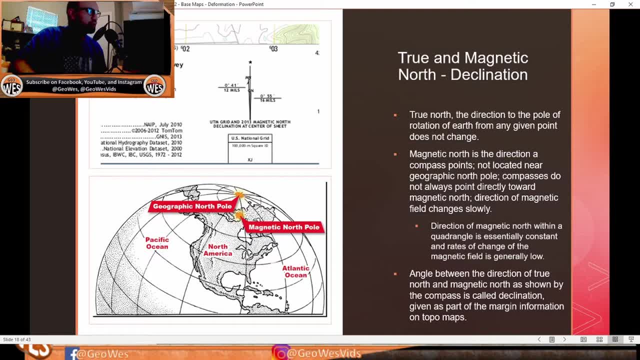 And we have geographic north Looks like right here, And then you have Minnesota Somewhere in here And that would represent, So it's a negative declination. Where I live, declination is about 7, 8 degrees. 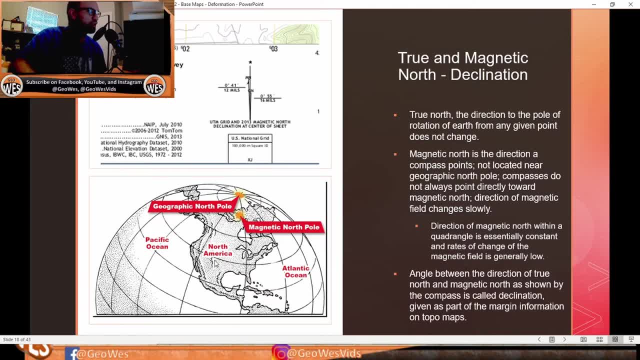 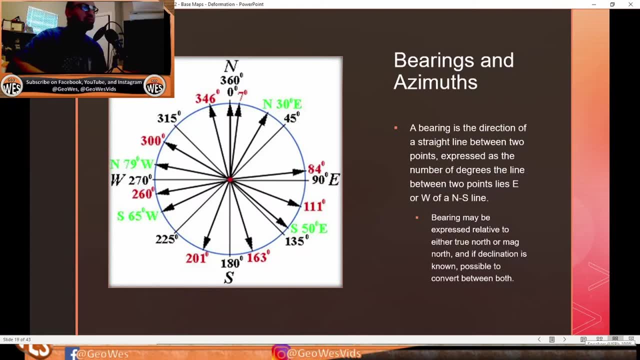 On Between, you know, geographic north and magnetic north, Somewhere right here. That's about 9 degrees difference. Bearing is an azimuth. A bearing is the direction of a straight line between two points, expressed as the number of degrees, the line between two points. 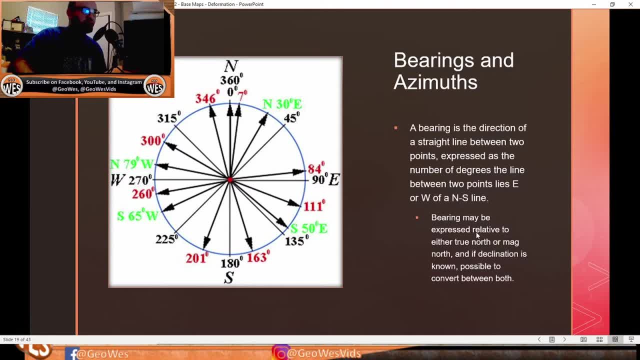 Lies east or west of a north-south line. The bearing may be expressed relative to either true north or magnorth And, if declination is known, possible to convert between both. And azimuth is basically 0 or 360,, 45,, 90,, 135,, 180.. 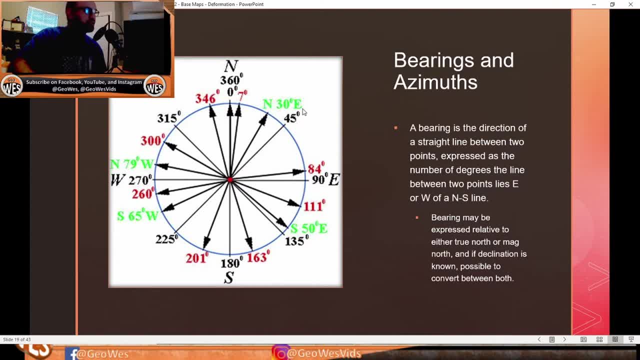 And then bearings is north 30 of 30 degrees of east. That's going to be 30 degrees in azimuth. This would be north 45 east. Of course that changes when you, you know you start getting down here. 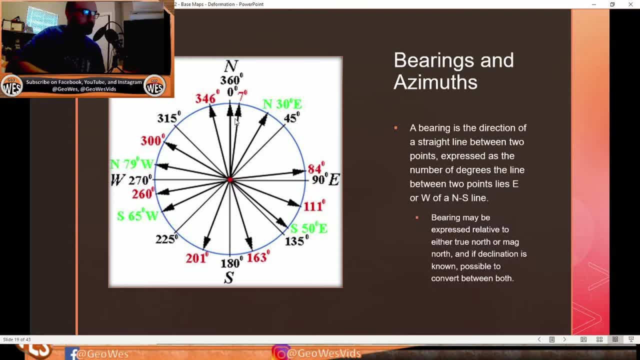 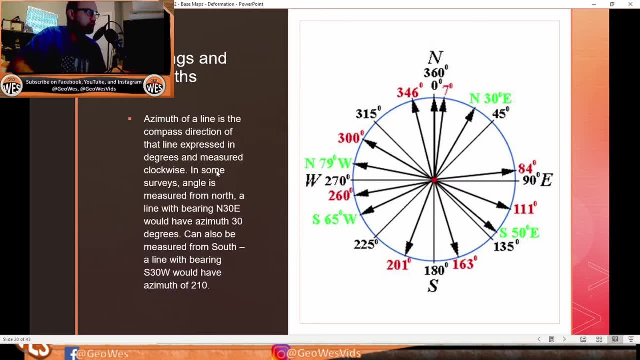 Or over here. you know, And I'll explain that right now, Azimuth of a line is the compass, direction of that line, expressed in the degrees and measured clockwise. In some surveys, angle is measured from north. A line with the bearing north 30, east would have azimuth 30 degrees. 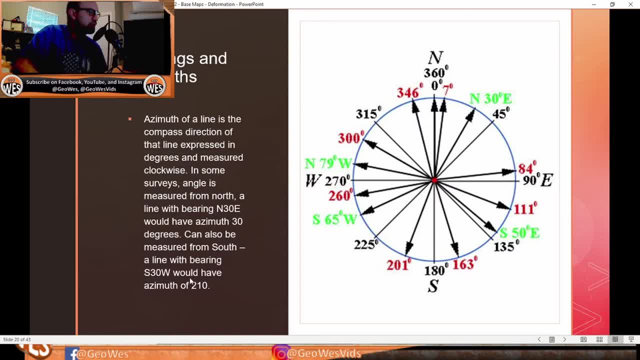 Can also be measured from south, A line with the bearing south 30 west. Sorry, Which would be about right here? Let's see, Yeah, about 210.. So right here would have 210 azimuth. Preparing a topographic profile. 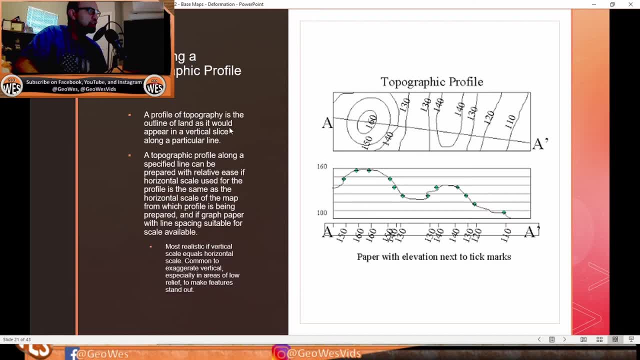 A profile of topography is the outline of land as it would appear in a vertical slice along a particular line. A topographic profile along a specified line can be prepared with relative ease if the horizontal scale used for the profile is the same as the horizontal scale of the map from which the profile is being prepared and if graph paper with line spacing suitable for scale available. 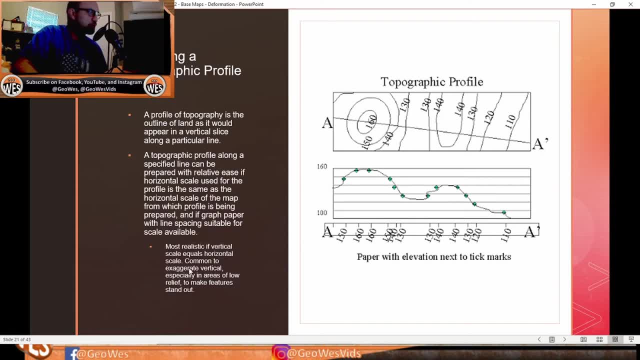 Most realistic if vertical scale equals horizontal scale. Common to exaggerate vertical scale, especially in areas of low relief, to make features stand out. And, as you can see, this is The map view. And then this is the With the cross-section line. 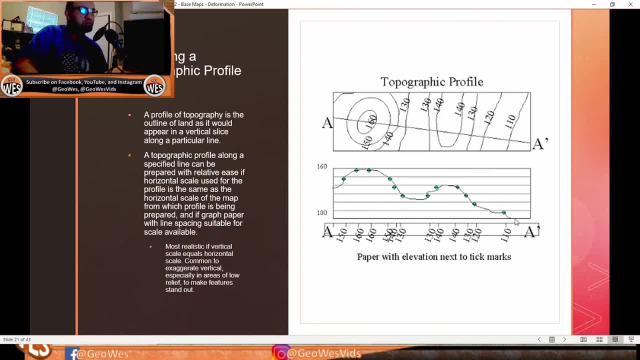 And then this is your topographic profile And we'll actually be going through an exercise. But it's good to master topographic profiles, especially if you're a young student, Because if you master topographic profiles before even doing a geologic cross-section, you know you're going to be ahead of the other students in your class. 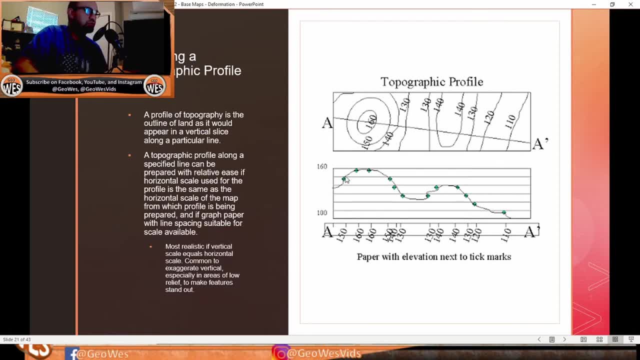 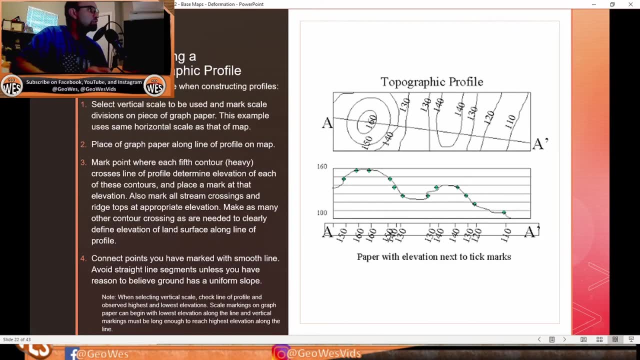 But I mean, if you're taking the ASBOG exam, it's still good to practice these, And hopefully you mastered cross-sections during your field camp. So, following this procedure, when constructing profiles, select the vertical scale to be used and mark scale divisions on a piece of graph paper. 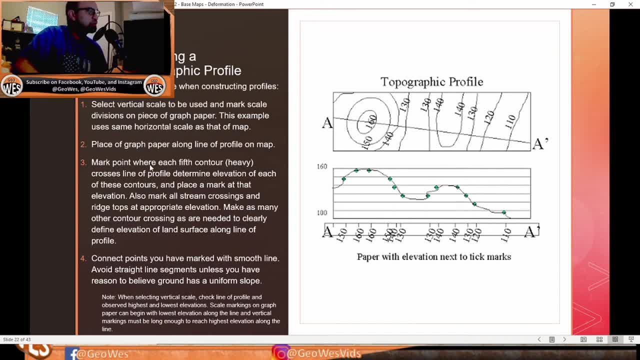 This example uses the same horizontal scale as that of the map. Place the graph paper along the line of profile on the map, which is this, the line of profile. I called it a cross-section line, but the line of profile Mark the. 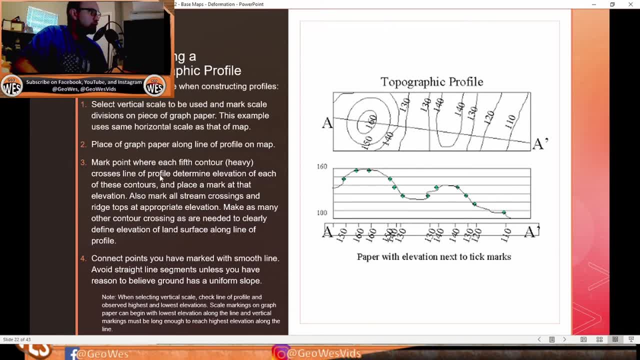 The point where each fifth contour or heavy contour- I called it a major contour line- Mark each fifth contour that crosses the line of profile, Determine the elevation of each of these contours and place a mark at that elevation. Also, mark all stream crossings and ridge tops at appropriate elevation. 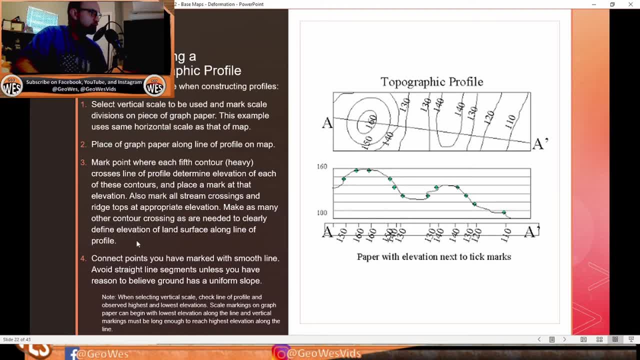 Make as many other contour crossings as are needed to clearly define the elevation of land surface along the line. The point where each fifth contour is marked is the line of profile. The point where each fifth contour is marked is the line of profile. You know you would mark 160,, 150,, 140,, 130,, 120,, 140,, 140,, 130,, 120,, 110, and that would give you you know your, your line, your profile. 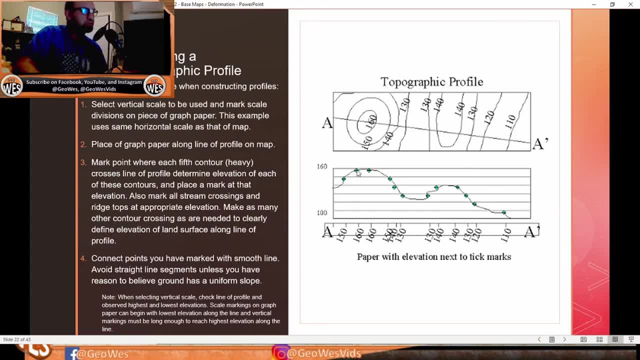 And you don't want to create angular lines between these points. You want to draw it as smooth as possible because that would be the most accurate profile And connect the points you have marked with a smooth line. Avoid straight lines Segment unless you have a reason to believe the ground has a uniform slope. 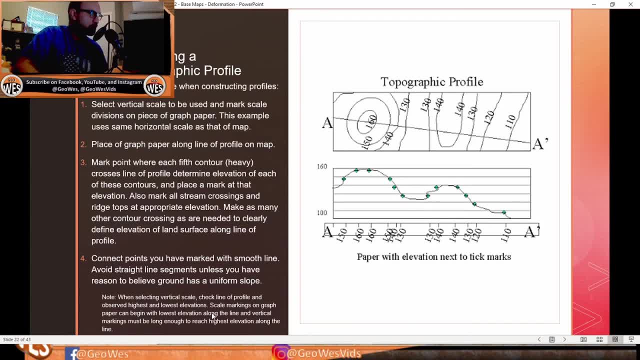 Note: when selecting vertical scale, check the line of profile and observe the highest and lowest elevations, which the highest and lowest are 160 and 110 in this particular profile. Scale markings on the graph paper can begin with the lowest elevation along the line. 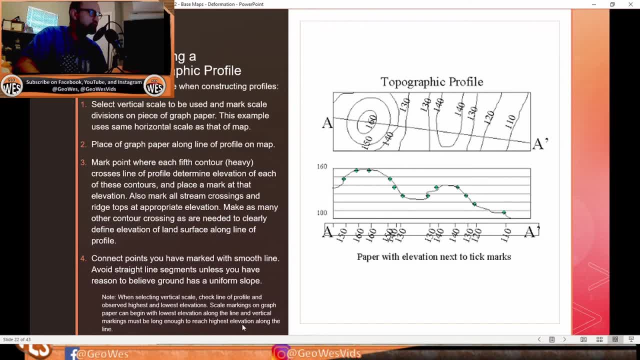 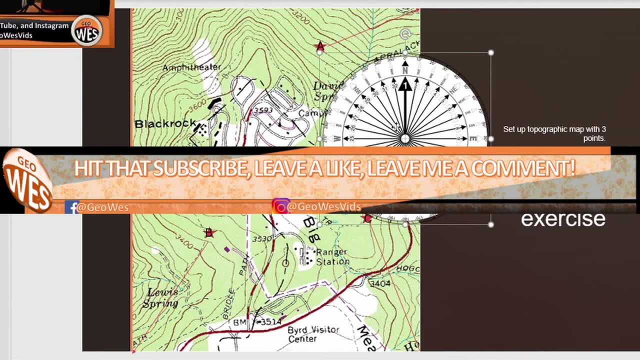 and the vertical markings must be long enough to reach the highest elevation along the line. All right, so let me exit out of this real quick. So we're going to do a little bit of work here. We're going to do a quick bearings exercise, and this isn't in complete order. 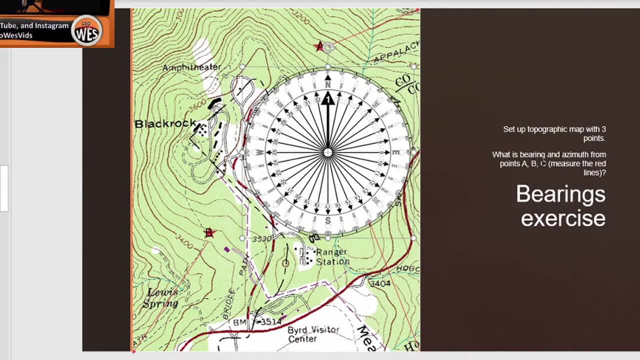 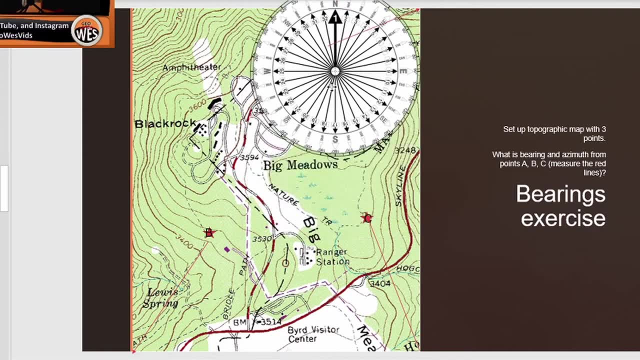 All right. so what we're doing is we're going to what is the bearing in azimuth from points A, B and C? Measure, basically measure the red lines that I've created. So A is about right here, So it kind of looks like: oh wow, I made it hard to see. 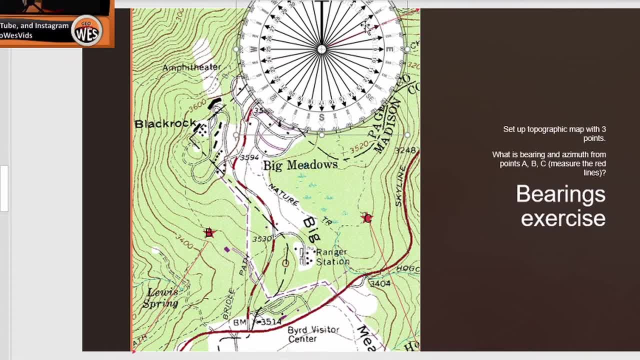 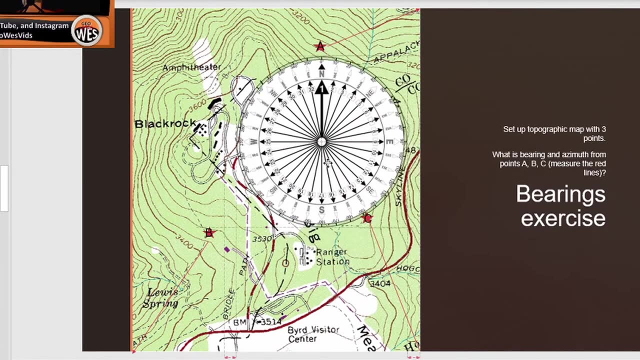 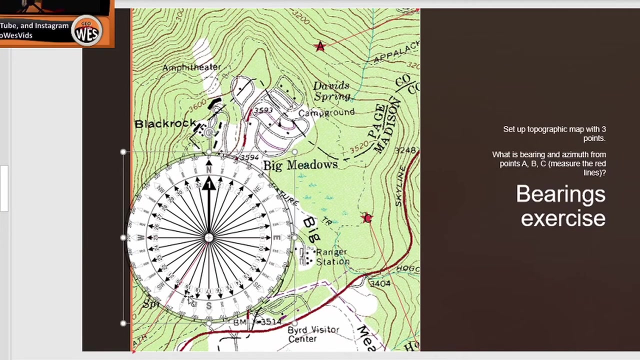 Okay, so the bearing of this particular line would be north seven east, north 67 east and in terms of azimuth, at 67.. So let's try B. B is about right there. Let's see south. what is that? 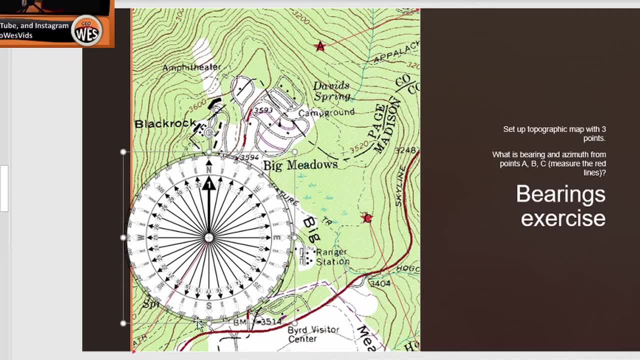 10,, 20,, 30,, 32.. South, 32, west, in a bearing And in terms of azimuth, you have let me see 7.7 east, north, 67 east and in terms of azimuth at 67.. 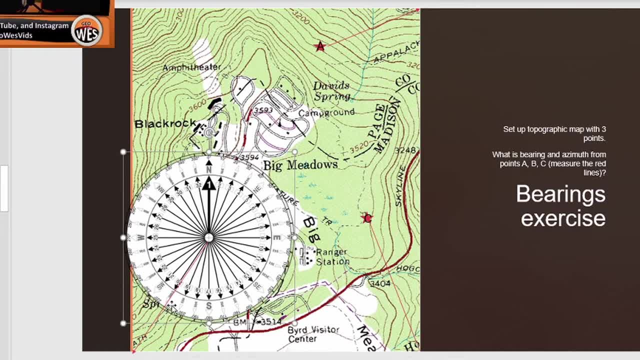 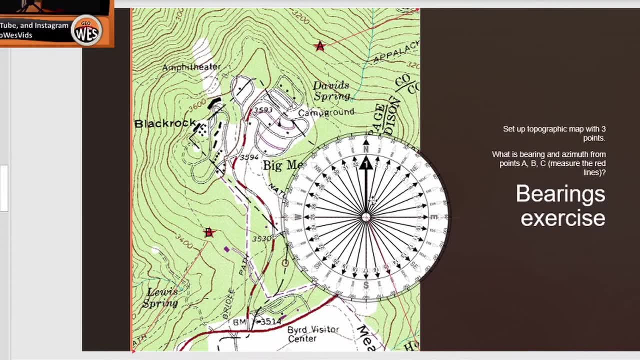 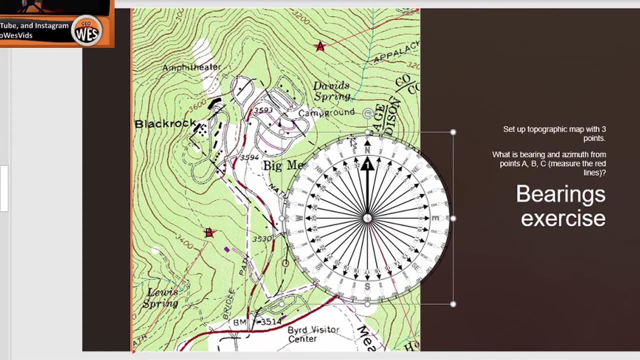 you have 200, what 12, something like that for azimuth notation. okay, and then, all right, so c? let's see, this is going to be south, that's what? 12? south, 12, east, and then, in terms of azimuth- and i personally prefer azimuth for this reason, because it can- 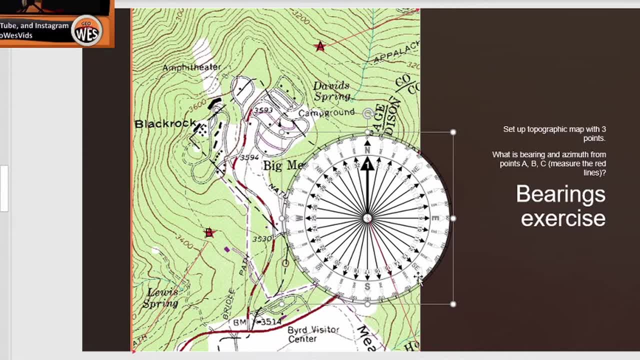 get a little confusing, but it's important to understand and be able to convert between the two notations. this is what: 158 degrees, something like that on azimuth. but it, like i said, it's important to practice this and understand and be able to convert if you're studying for the 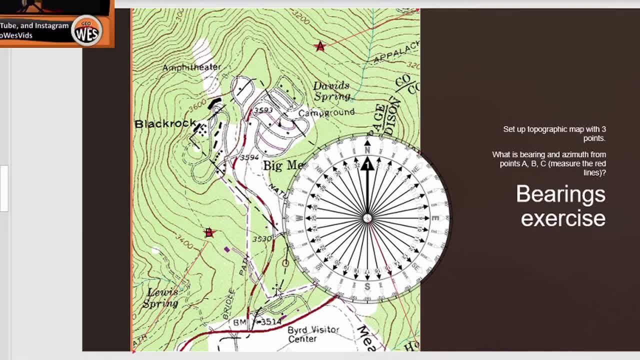 asbog, or i mean, if you're a student and getting into geoscience, you definitely want to understand how to, how to- uh, definitely, uh, you know- convert between the two and be able to understand how to measure these lines. all right, so we're going to be working on. 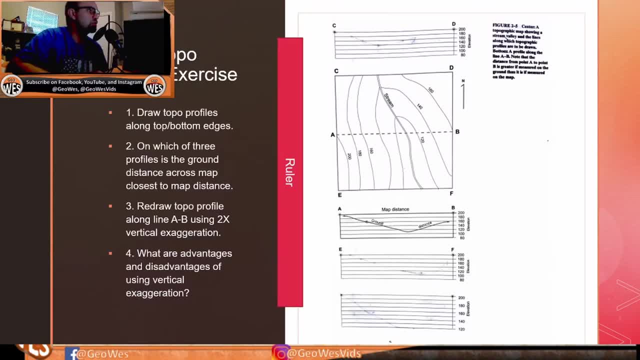 an exercise right now, another one. so it's a draw topo profile exercise and i'm going to try and do it the best i can. uh, it's not going to be perfect because i'm doing it on powerpoint, but uh, draw the topo profiles along the top and bottom edges of each of these cross sections. 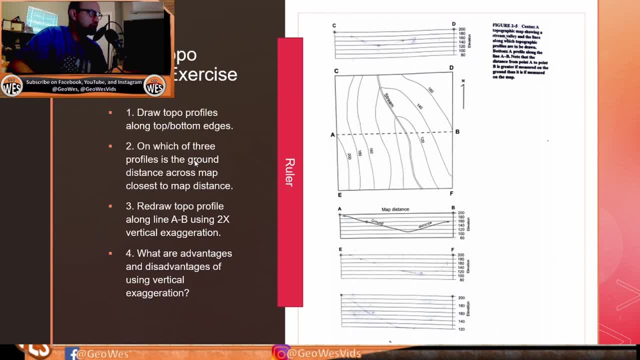 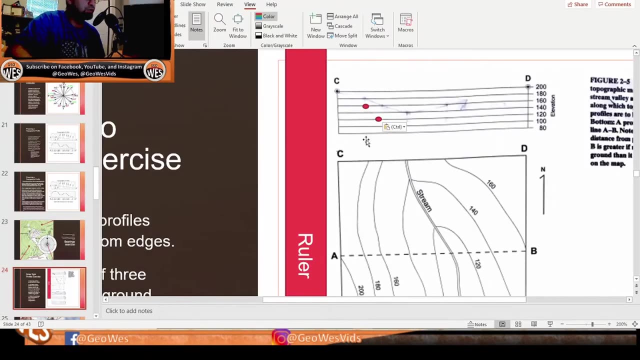 on which of three profiles is the ground distance across map closest to the map distance? redraw the topo profile along line a and b using two times exaggeration, and what are the advantages and disadvantages of using vertical exaggeration? so this is actually 180, okay, so this one should be. 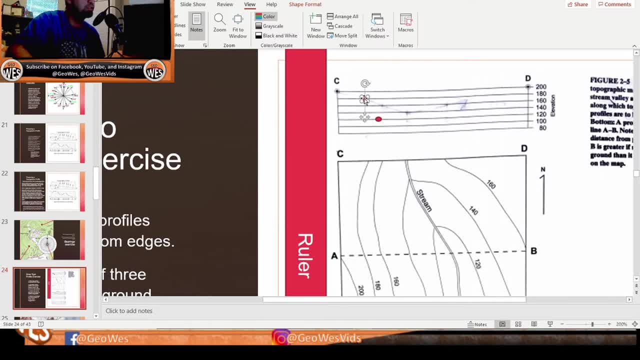 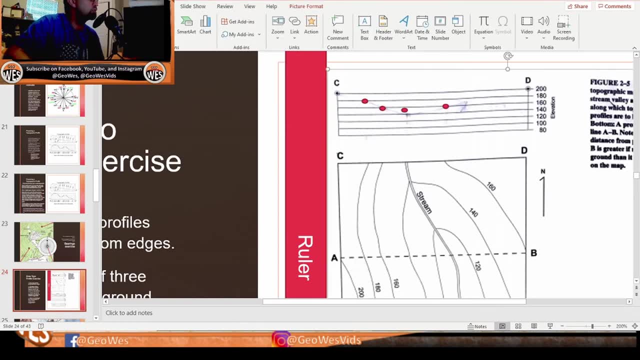 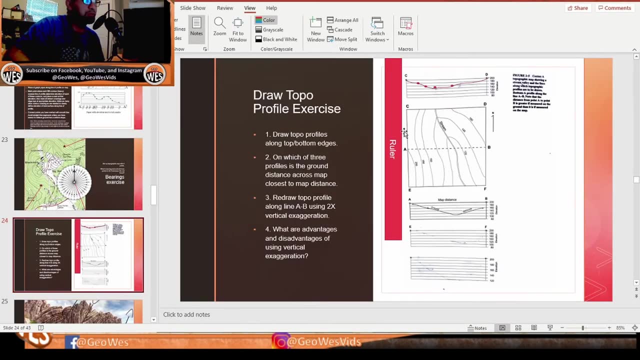 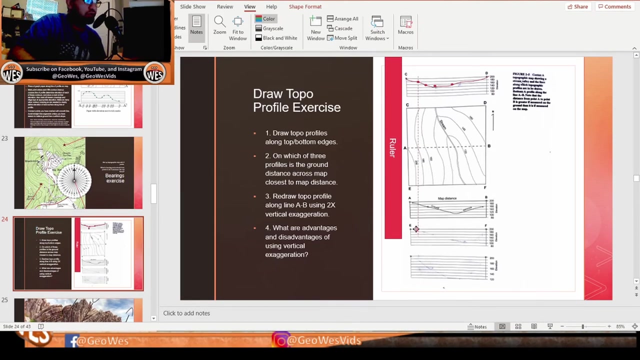 a little bit higher. put it right there. let's see 160. so now we're going to try and draw this- and this is the fun part, because i don't know if i can draw this. okay, so that's our topo profile for cd. it's kind of a pain in the butt. okay, they did a and b for us. e and f is going to be. that's 200. 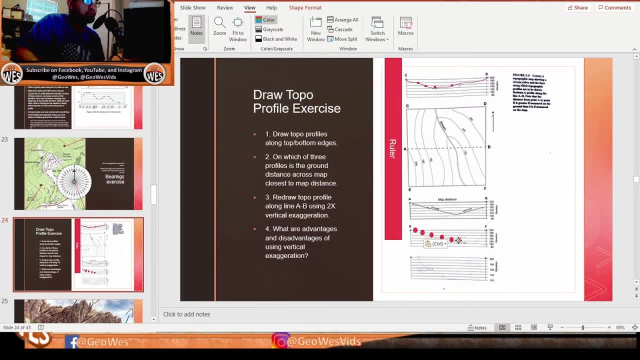 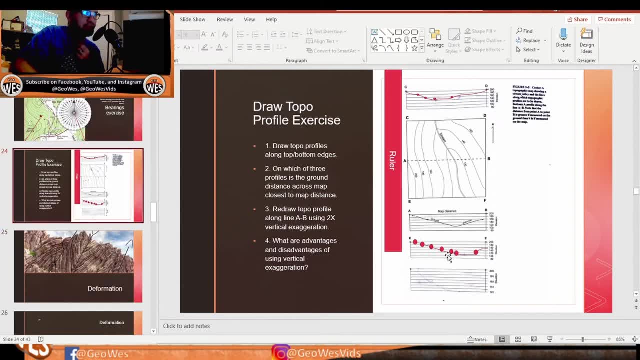 right here, and then we'll have a stream point and it'll probably be a little bit lower than 120. so let's draw this real quick and obviously it will look much better than that. if i could actually freehand this zoom in- well, i guess i can't, that's stupid, um. so yeah, this would look. this would actually have. 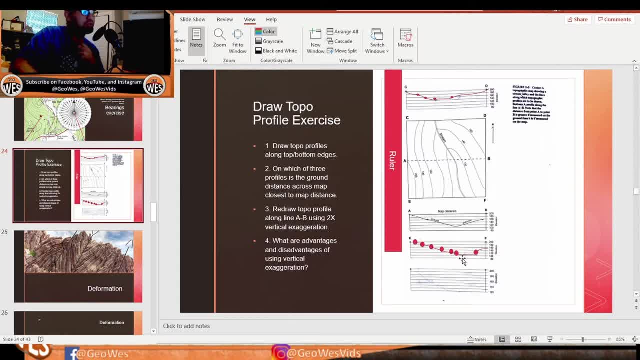 a little bit more of a valley. i can't draw a valley for some reason, but uh, this would have a little bit more of a valley and then it would increase to about 140. so this would be. this line would be a little bit lower to about right right here. so that's basically with the vertical scale. 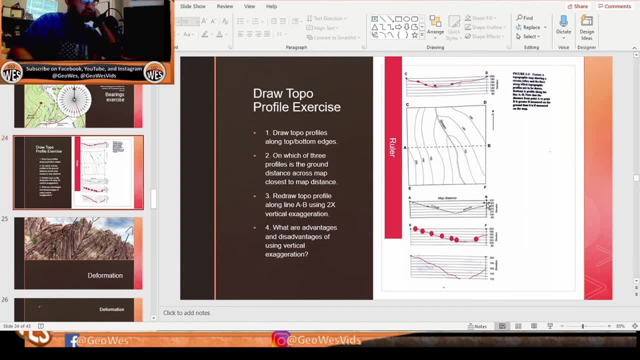 exaggerated. this is what it looks like, not exaggerated. this is what it looks like exaggerated, as accurate as i can get it, but uh, you know it brings out the relief a lot more. when you exaggerate the vertical scale, typically in a geologic profile, you'll want to um, typically. 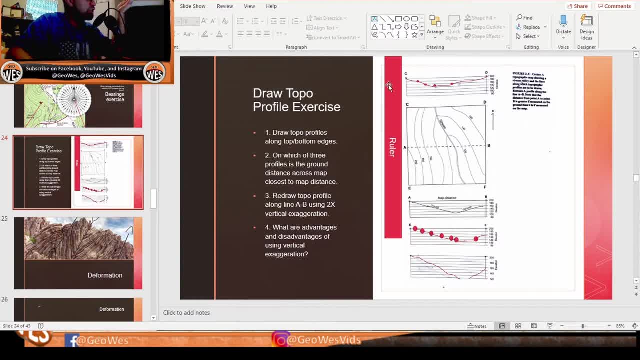 your professor will ask you to um, what's it called to? there's a, there's a way to calculate it. i'm not going to include in this episode, we'll probably get into it later- but there's a way to get the perfect uh vertical scale for your geologic cross-section, um to where you're not exaggerating the relief. 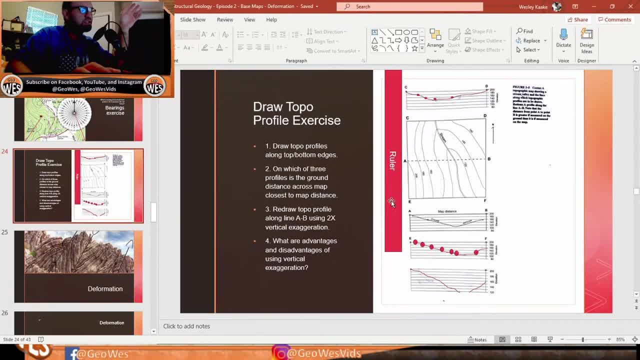 because typically, you know, in places where you're exaggerating and you're doing a cross-section, you know you're going to have terrain. you typically want to not exaggerate your vertical, not even at a one-to-one. it's actually less. you know it depends on the, the relief in your area. 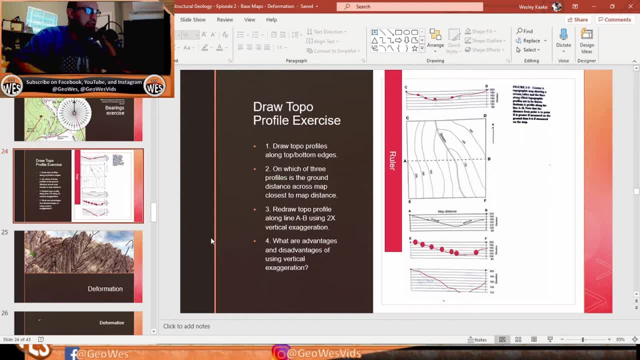 so, anyways, uh, i tried to describe, uh explain that as best as i could using technology, but you know, i hope you guys understood. if there's issues, i'll redo this. um, i highly recommend you buy this book and do you know the this practice and practice? topographic profiles in general? 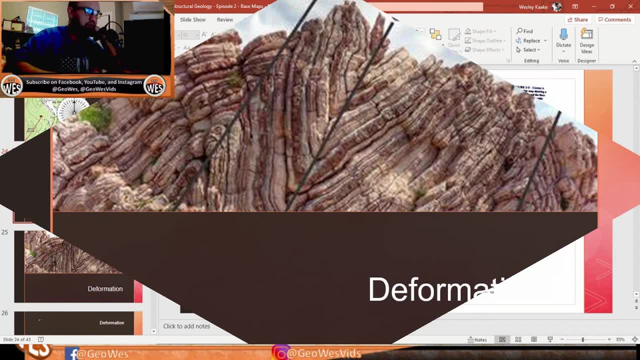 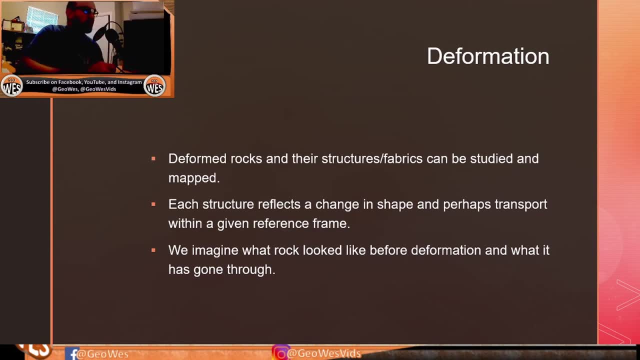 create your own by looking at topographic maps. all right, so now we're going into deformation. so deformation is uh, okay. deformed rocks and their structures or fabrics can be studied and mapped. each structure reflects a change in shape and perhaps transport within a given reference frame. we imagine what. 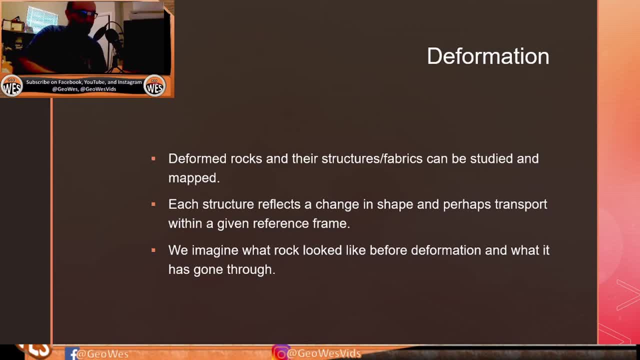 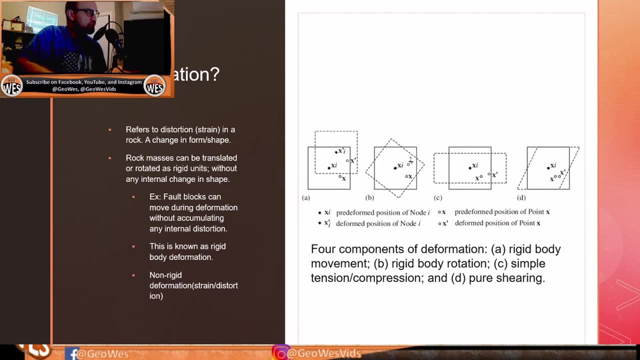 a rock looked like before deformation and what it has gone through. so what is deformation? it refers to the distortion or strain in a rock. it's a change in form or shape. rock masses can be translated or rotated as rigid units without any internal, internal change in shape. so an example is a fault block can move during deformation without accumulating any. 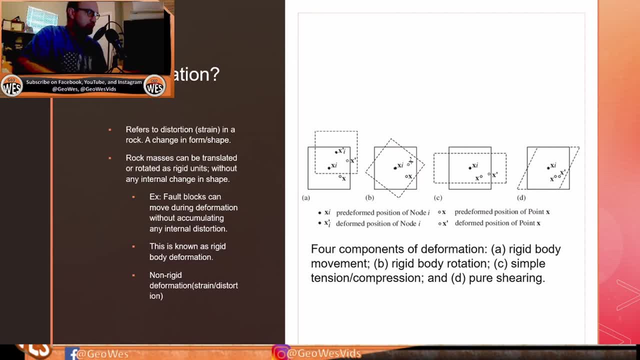 internal distortion. this is known as rigid body deformation. non-rigid deformation is strain or distortion, which means an internal shape change. so this is translation you: just it's keeping the same shape, it's just, uh, moving to a different spot. this is rotation, uh, this is uh. deformation is the transformation from an initial to final geometry, geometry by. 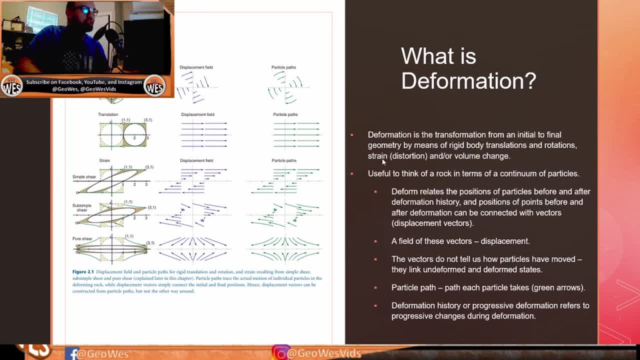 means of rigid body translations and rotations, strain distortion and or volume change. it's useful to think of a rock in terms of a continuum of particles. deformation relates to the positions of particles before and after deformation. history and positions of points before and after deformation can be connected with vectors- displacement vectors. 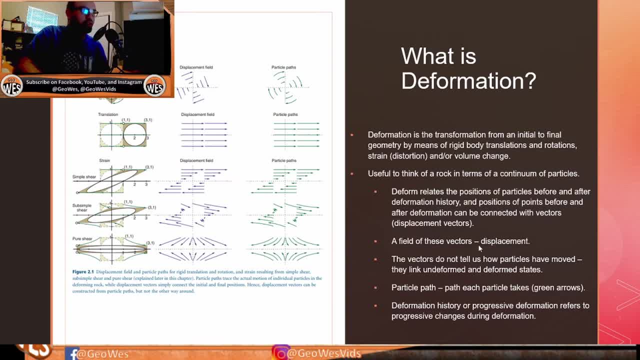 a field of these vectors- displacement filled. the vectors do not tell us how particles have moved. they link undeformed and deformed states. the particle path- path each particle takes is the green arrows, as you can see here. this is displacement fields. deformation history or progressive deformation refers to progressive changes during deformation. so components of 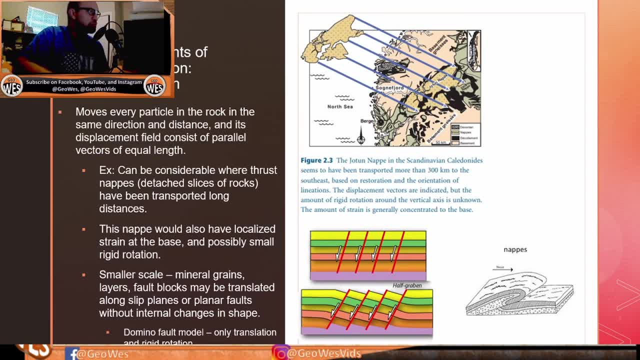 deformation translation. it moves every particle forward and backward in the same direction and distance, and its displacement field consists of parallel vectors of equal length. an example can be considerable, where thrust naps, the detached slices of rocks, have been transported long distances and this, uh, this figure shows. you know what this is a nap. 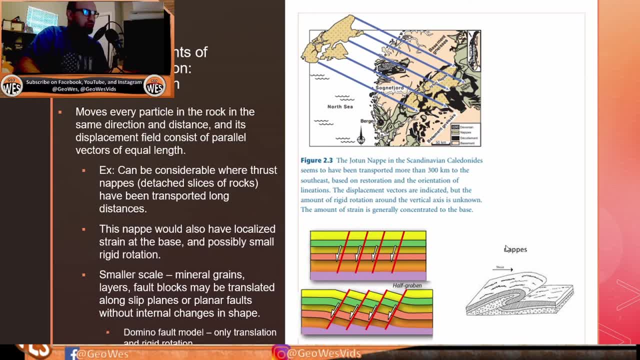 it's typical in compressional and reverse thrust. and, um, yeah, reverse thrust faults. uh, this nap could. it's typical in compressional and reverse thrust, but it's only useful for the. it's typical in compressional and reverse thrust. it's only used with a larger carbon. 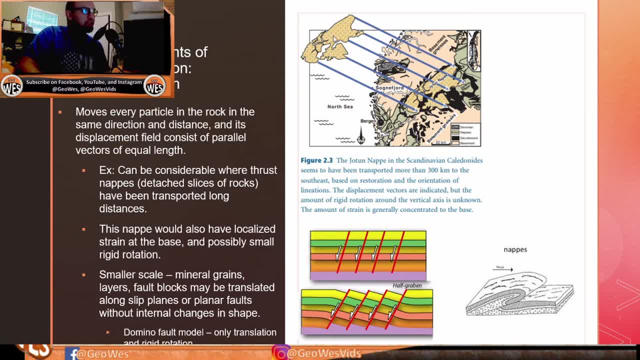 ion that can act as a пуbert and to achieve it. you know, you have this big, very big body of rock and it's slowly being moved over millions of years and and now it's over here. and where is this? if you don't look at the board, you can see it here in its first shape. and then you have this. 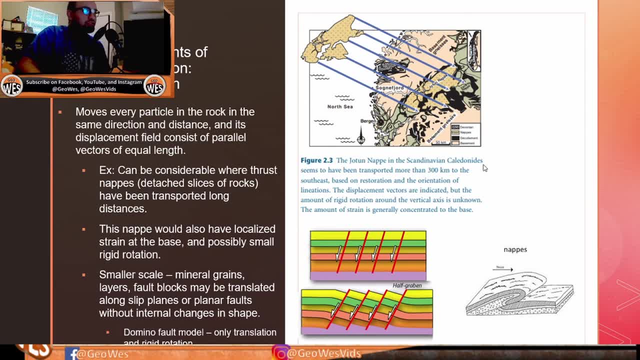 nap in the scandinavian cala don't needs. i don't know how to say that, but uh, yeah, it started off over here and it's been pushed, and now it's over here and this uh looks like a mountain range. so smaller scale mineral grains, layers, fault blocks may be translated along slip planes or 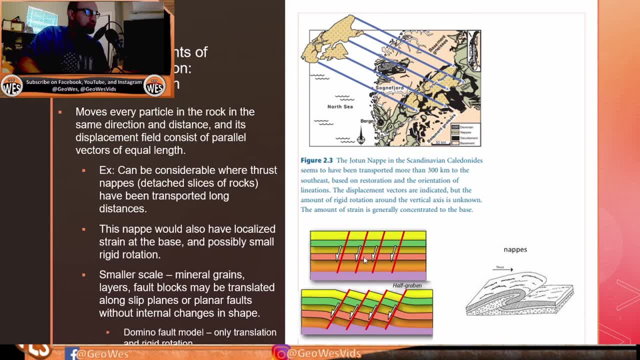 planar faults without internal changes in shape, as you can see, the domino fault model, and we'll- i believe we'll- go deeper into that, but it's a normal fault, it's a characteristic. in a normal fault area you only have translation or movement, you know. 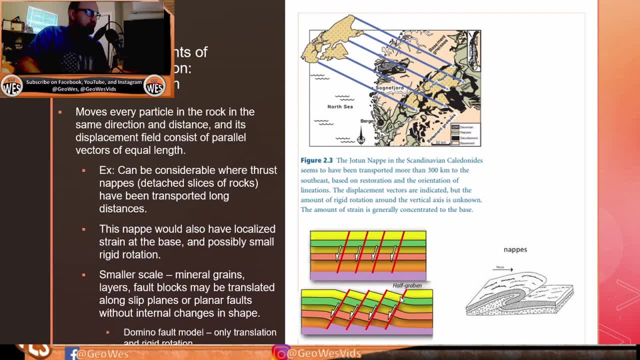 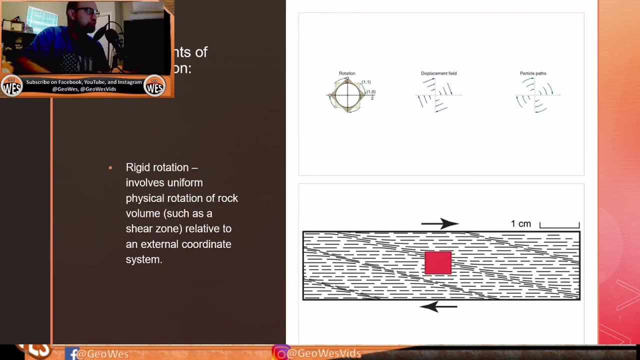 you know it starts like this and then it moves like this and rigid rotation, so it slightly rotates and translates down and you can see that it does that at every fault block. so rotation, rigid rotation, involves uniform physical rotation of rock volume, such as a shear zone relative to an external coordinate system and yeah, as i said earlier, it just rotates, you know. 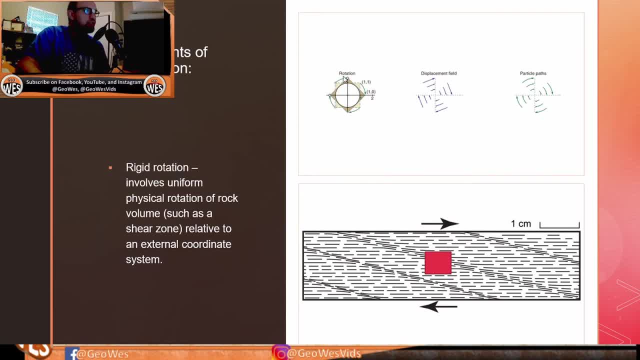 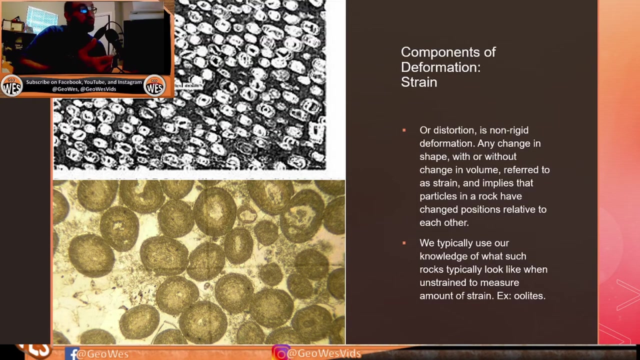 it starts off like this: the light brown and rotates and you use basically x, y axes to put so this one starts at negative, one and and one it comes to zero and one. so components of deformation: strain or distortion is non-rigid deformation, which means you have an internal structure change. 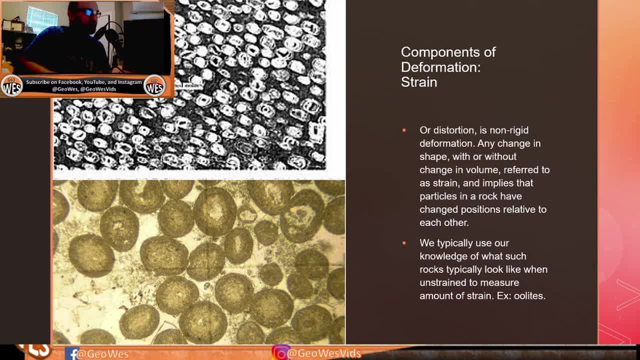 any change in shape, with or without change in volume, referred to as strain and implies that the particles in a rock have changed positions relative to each other. we typically use our knowledge of what, such what, what the rocks typically look like before going under strain to measure the amount of strain. So an example is what you see on the left is 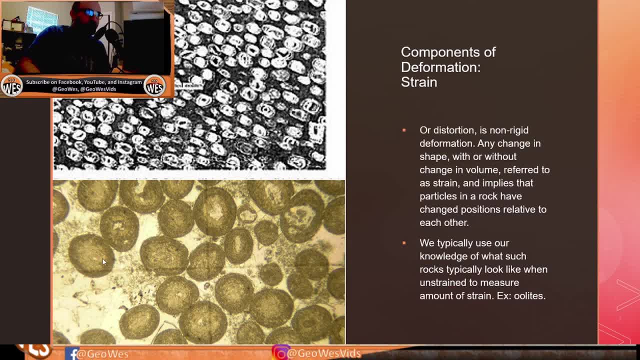 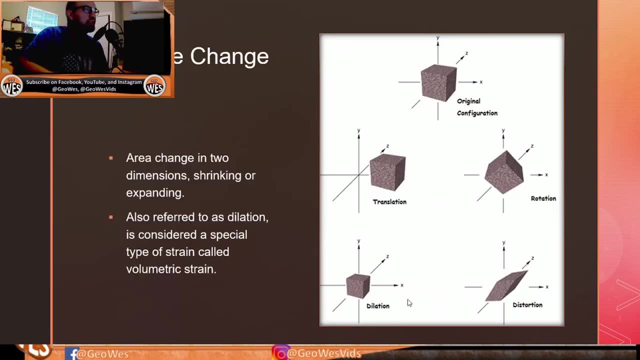 an oolite. It's typically not perfectly spherical, but it's pretty much visualized spherical perfectly. So obviously, if these become elongated, you can measure the amount of strain that these oolites have gone through. A volume change is an area change in two dimensions, shrinking or 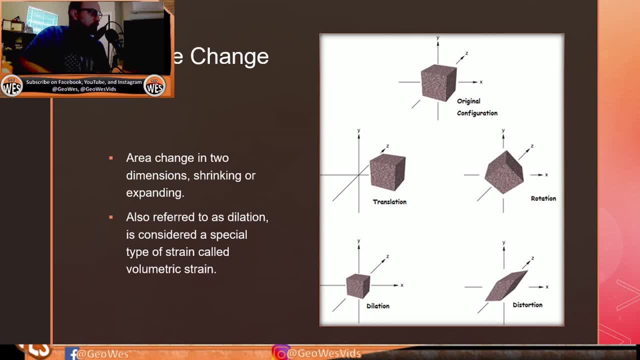 expanding. It's also referred to as dilation and it's considered a special type of strain called volumetric strain, And this is another way to visualize translation. This is the original configuration. It's been moved to the right and then rotation. It's been gently, you know, rotated and then 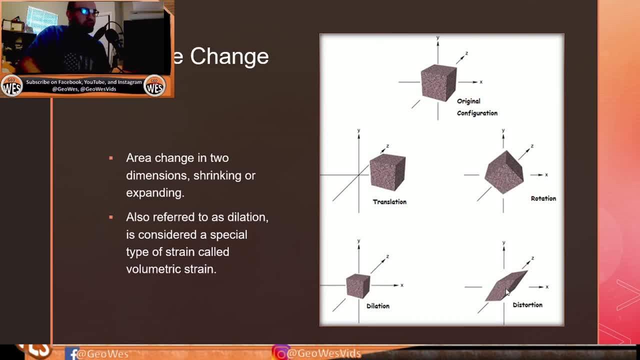 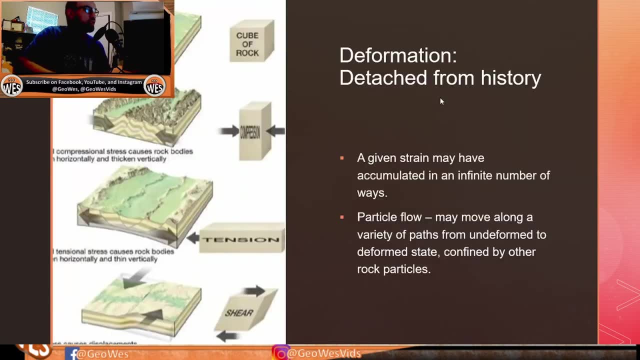 dilation just basically means the shrinking and distortion. As you can see, it changes significantly in shape. It's shrinking and then it's dilating. It changes significantly in shape. It's shears from the original configuration, Detached from history, A given. 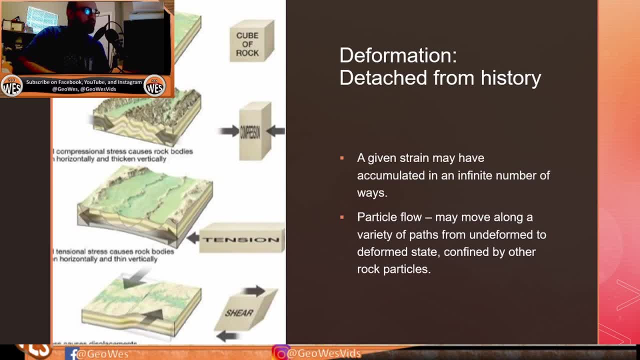 strain may have accumulated in an infinite number of ways. Particle flow may move along a variety of paths, from undeformed to deformed states confined by other particles, And this is another way to visualize it. This is your basic, your starting point: cube of rock when it undergoes compression. Obviously you have. 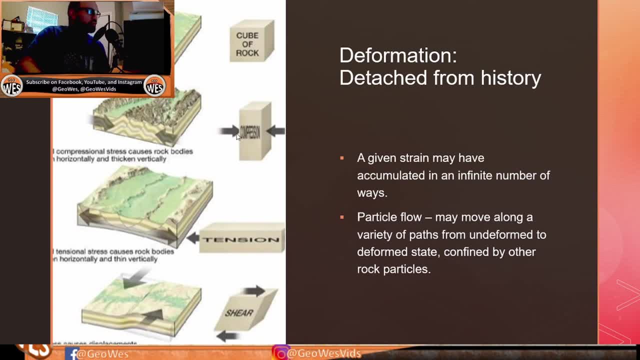 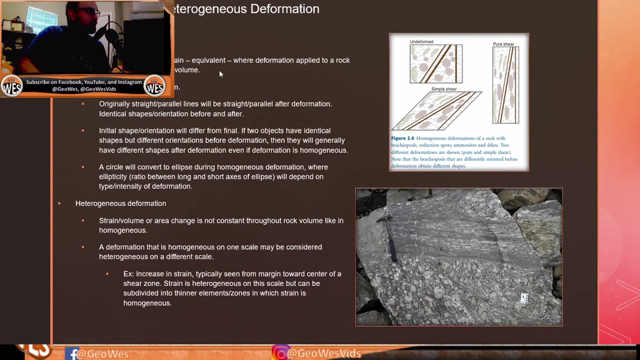 it the height increase vertically but the length decrease horizontally. in this this cube Tension pulls or elongates the cube of rock, so it increases horizontally or is elongated and then vertically shortens. So homogenous versus heterogeneous deformation. Homogenous deformation of strain is equivalent where deformation 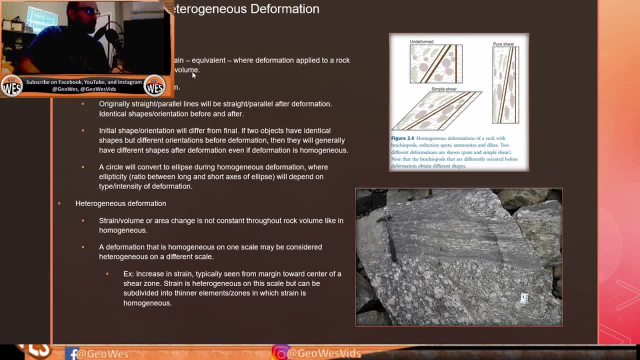 applied to a rock volume is identical throughout the rock volume, Rigid rotation translation. So no internal change in the in the in the rock. Originally straight parallel lines will be straight parallel after deformation. Identical shapes: orientation before and after. Initial shape orientation will differ from the final If the two objects have identical. 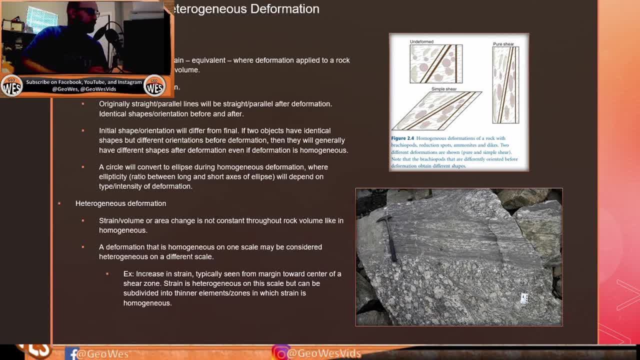 shapes but different orientations before deformation, then they will generally have different shapes after deformation, even if the deformation is homogenous. Circle will convert to an ellipse during homogenous deformation, where ellipticity- the ratio between the long and short axes of the ellipse will depend on the 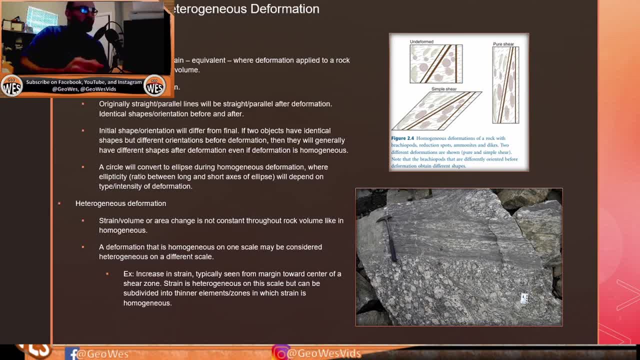 type and intensity of deformation And heterogeneous deformation. the strain volume or area change is not constant throughout the rock volume, like in homogenous. A deformation that is homogenous on one scale may be considered heterogeneous on a different scale. Increase in strain, typically seen from the margin toward the center of a shear zone. As you can see here, this is a shear. 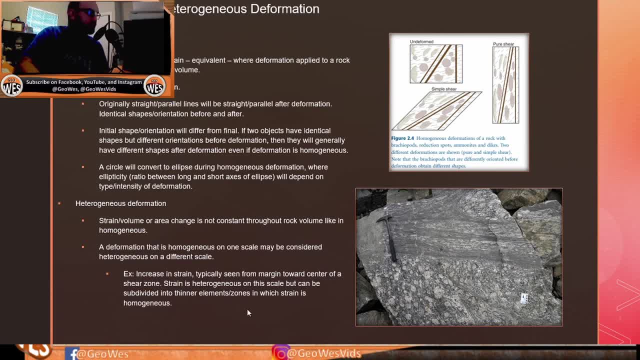 zone. Strain is heterogeneous on this scale but can be subdivided into thinner elements, zones, and which strain is homogenous. So a certain particle may have just been, you know, rotated or translated From here, you know, from how we're seeing it from this scale, you know it's. 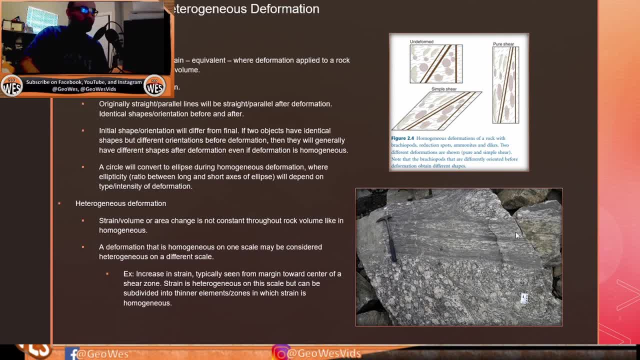 it's definitely heterogeneous. It's a- both heterogeneous and heterogeneous. It's a bunch of different. well, it's a. it's a volume change And undeformed. this is a good little figure that I like, and we'll get into what simple and pure shear mean. 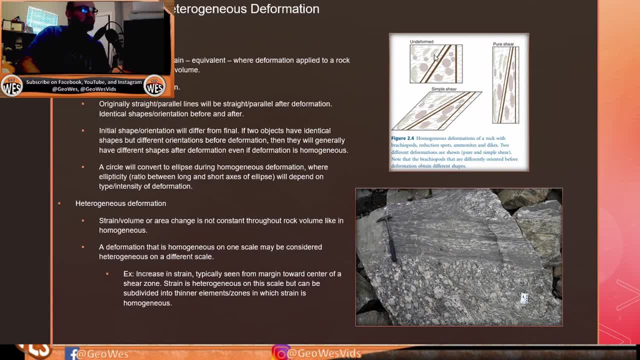 but basically you know you have your undeformed, what it looked like before deformation, and along this shear zone right here, and then you know it becomes elongated, the shear zone During pure shear, and these kind of change, uh, the fabrics change orientation as well as the uh. 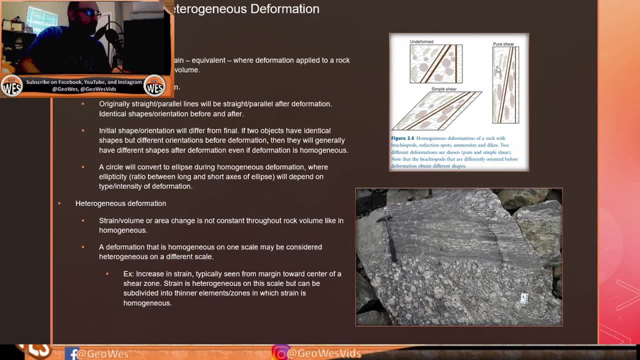 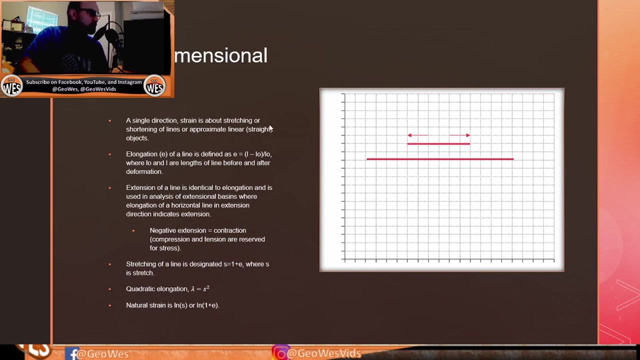 these fossils, uh, brachiopads- sorry, brachiopods- They become kind of elongated, they change, so you have a little bit of heterogeneous deformation there, and same thing with simple shear. they change, not necessarily their orientation, but they definitely become elongated. Okay, so one dimensional strain, a single direction strain, is about stretching or shortening of lines. 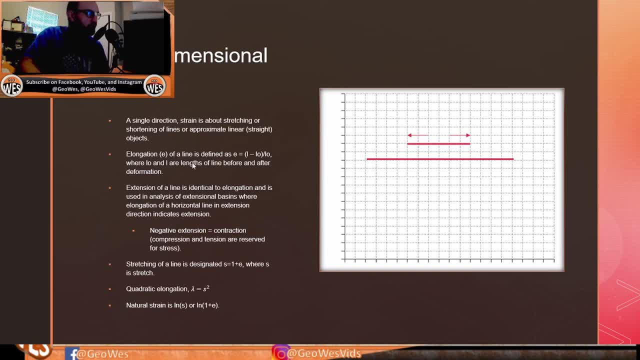 or approximate linear straight objects. elongation or E- and we won't go too much into this math because it's not important for the ASBOG, but uh, elongation of a line is defined by E. equals length minus the original length divided by the original length, Where LO and 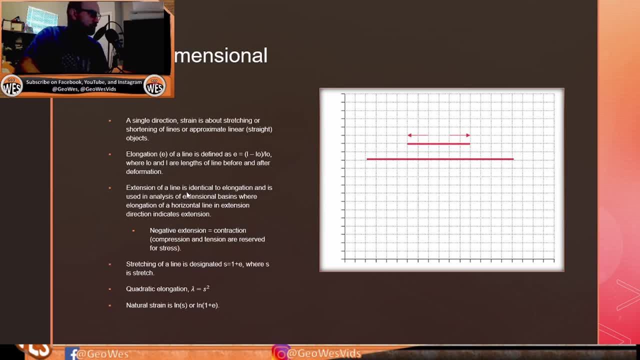 L are lengths of line before and after deformation. Extension of a line is identical to the elongation and is used in an analysis of extensional basins, where elongation of a horizontal line in an extensional direction indicates extension. Negative extension is contraction and that's related to compression and tension, which is reserved for stress. 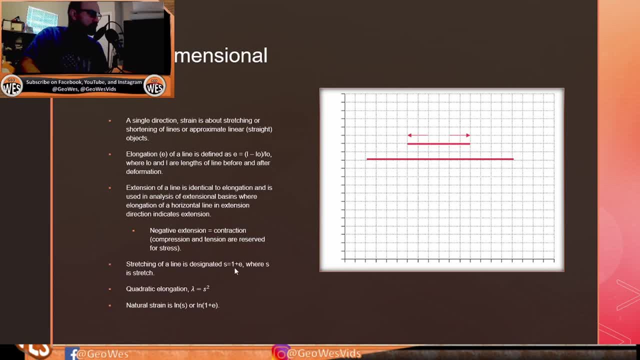 Stretching of a line is designated by S equals 1 plus E. where S is stretched, Quadratic elongation is that symbol equals S squared or stretching squared. Natural strain is LN S or LN 1 plus E. Two-dimensional strain. observations of strain in planes or sections. 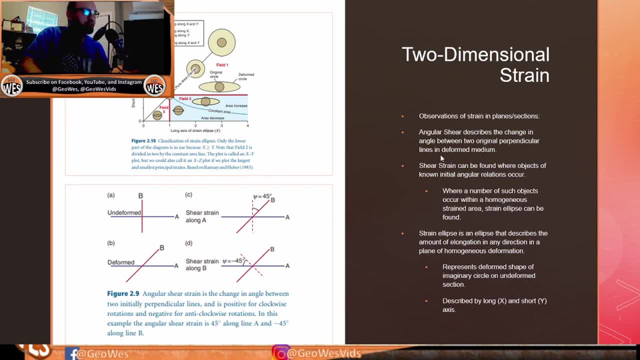 Angular shear describes the change in the angle between two perpendicular lines in the deformed media. An angular shear. is this symbol right here. I couldn't find it on PowerPoint, but yeah, it's this symbol. Shear strain can be found where the objects of unknown angular relations occur. 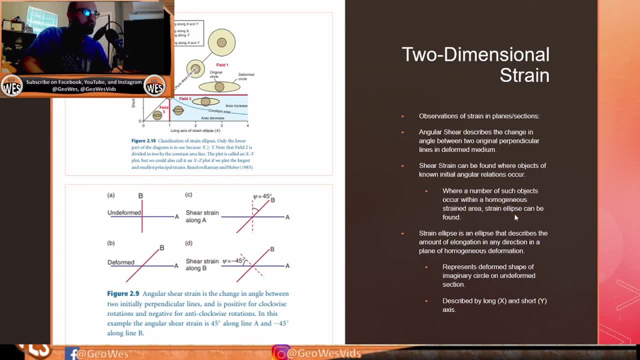 Where a number of such objects occur within a homogenous strained area, the strain ellipse can be found. The strain ellipse is an ellipse that describes the amount of elongation in any direction in a plane of homogenous deformation. represents the deformed shape of the imaginary circle. 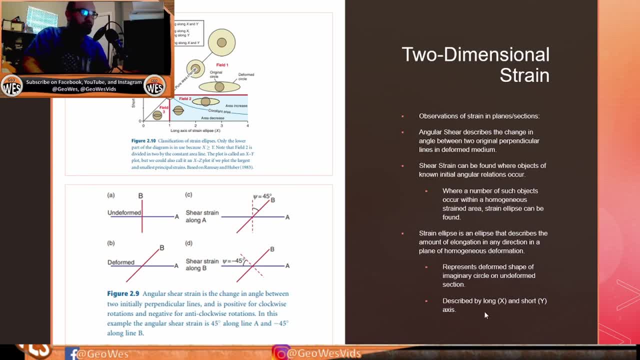 The strain ellipse can be found on the undeformed section and it's described by the long and short axis, or X and Y axis. So this is your original strain circle at this point, And then as you get into elongation- or actually this is dilation, right. 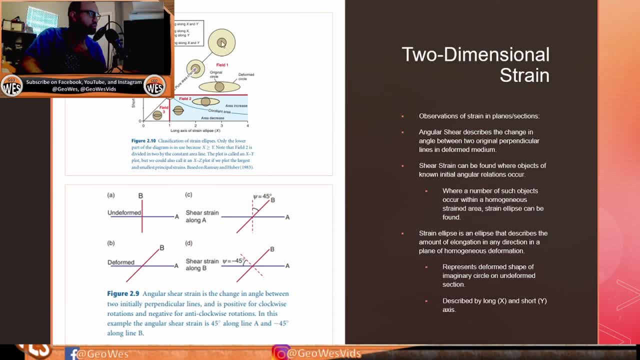 No, this is expansion. Field 1 is going to be expanding on this pier Area change. It's expanding out. If you have an elongation in the X direction, then obviously it becomes this one in the background. This is your original circle. 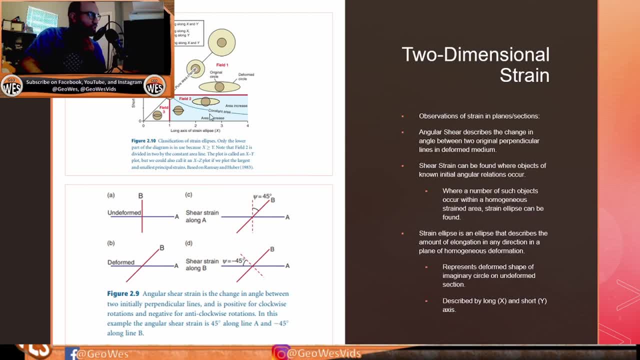 This is your deformed circle And then an area decrease, it shortens vertically and elongates horizontally. And then this one obviously shortens horizontally, I mean vertically, and kind of increases Horizontally. And then field 3, it looks like it decreases in both. 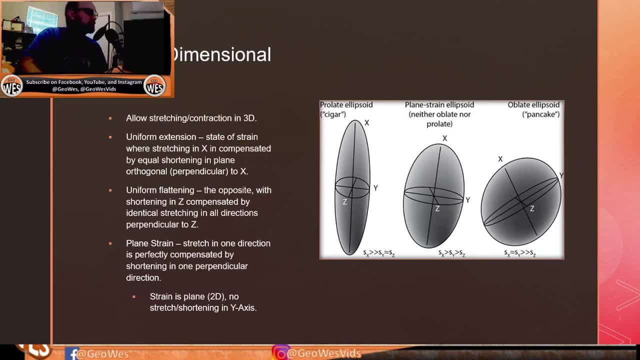 Horizontally and vertically. Three dimensional strain: It allows stretching and contracting in three dimensions. Uniform extension: the state of strain where stretching in X is compensated by equal shortening in the plane orthogonal or perpendicular to X. Uniform flattening: the opposite. 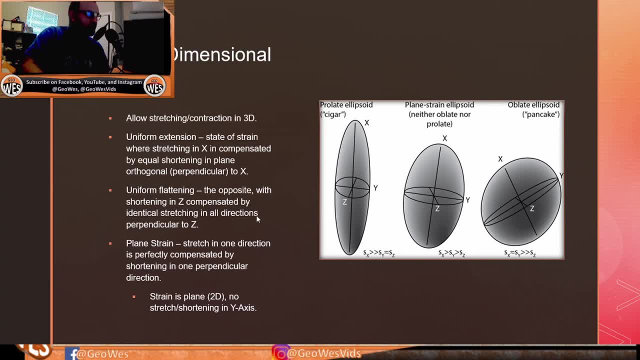 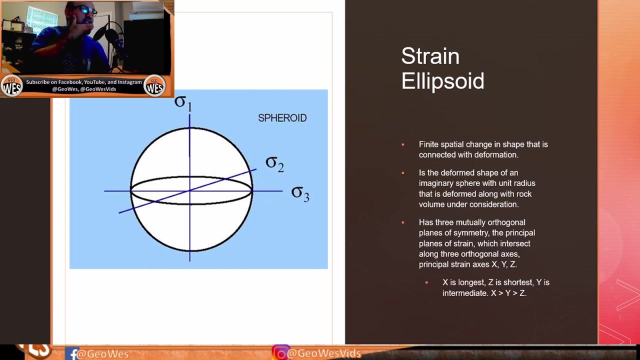 With shortening And then plane strain is stretched in one direction. that is perfectly compensated by shortening in one perpendicular direction. The strain plane is two dimensional: no stretching or shortening in the Y axis. The strain ellipsoid, which is what we just saw in the previous slide, is a finite spatial change in shape that is connected with deformation. 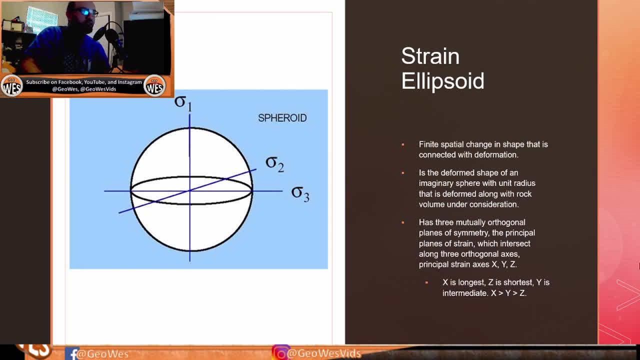 And, as you can see, sigma 1,, sigma 3,, sigma 2.. So the strain ellipsoid is the deformed shape of an imaginary sphere with unit radius that is deformed along with the rock volume under consideration. It has three mutually orthogonal planes of symmetry, the principal planes of strain, which intersect along three orthogonal axes: X, Y, Z. 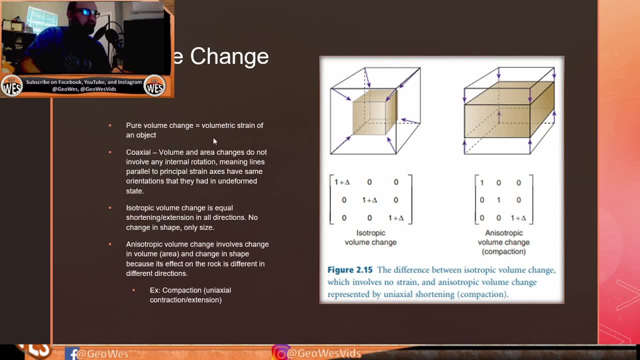 The volume change per volume change equals volumetric strain of an object, Coaxial. The volume And area changes do not involve any internal rotation, So meaning lines parallel to principal strain axes have deform, have the same orientations that they have they had in the undeformed state. 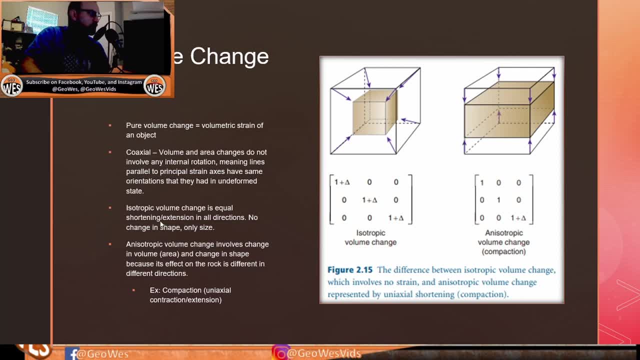 Isotropic volume change is equal in equal shortening and extension in all directions. No change in shape, only size. So this is your isotropic right here. An isotropic volume change involves change In the volume or area, In the area In the volume. 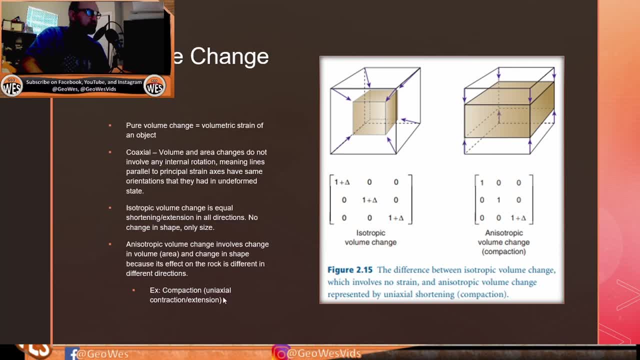 change in shape because its effect on the rock is different in different directions. so compaction. so this is an anisotropic. as you can see, there's basically just a compression that changes the, the height of the square, the original square. sorry cube, it changes the height of the cube. 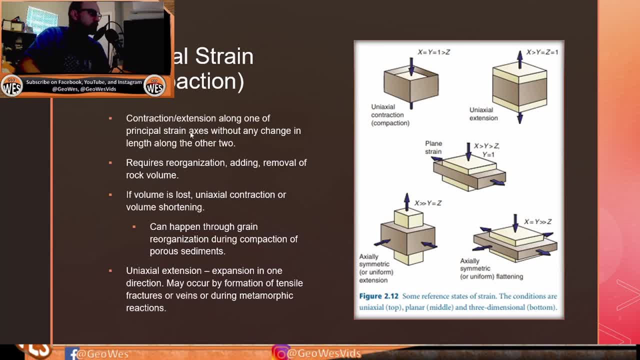 uniaxial strain or compaction, contraction and extension along one of the principal strain axes without any change in the length along the other two requires reorganization, adding or removal of the rock volume. if volume is lost, uni uniaxial contraction or volume shortening can happen. 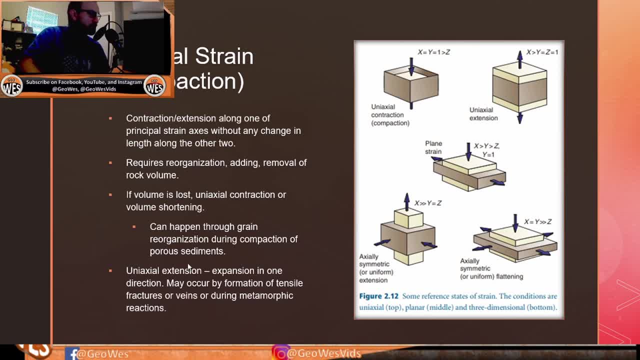 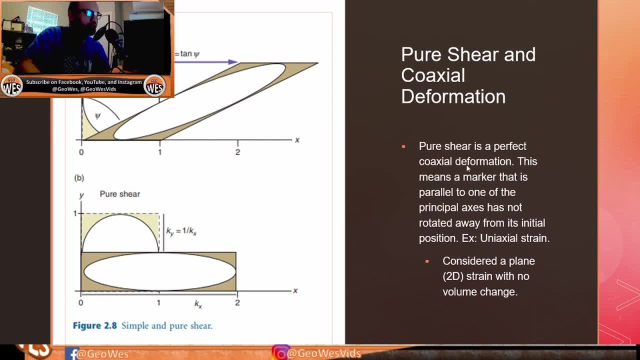 coaxial deformation. so pure shear is a perfect coaxial deformation. this means a marker that is parallel to one of the principal axes has not rotated away from its initial position. so an example is uniaxial strain considered a plain strain with no volume change. so this is pure shear.